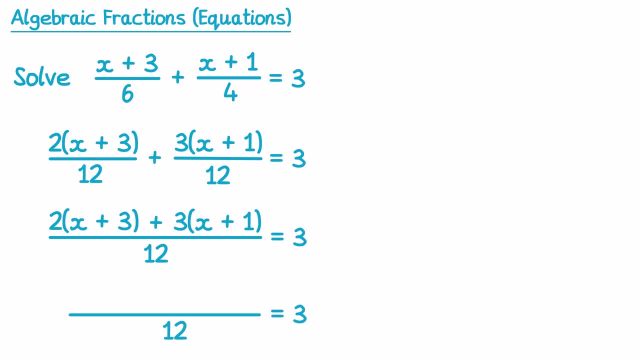 multiply by 2 lots of x plus 3, and then we're going to expand the numerator here. So we've got 2 lots of x, that's 2x. 2 lots of positive 3,, that's positive 6, then we've got a positive 3. 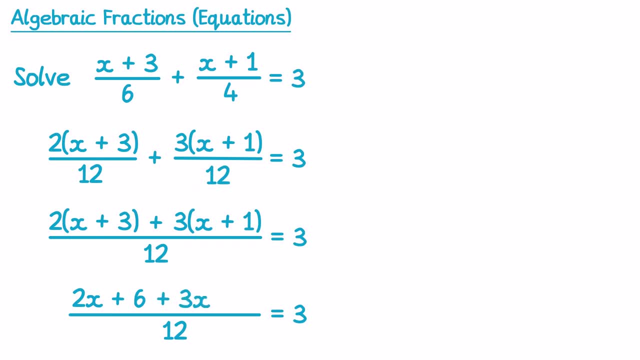 times x, that's positive 3x, and then positive 3 times positive 1,, that's positive 3.. We can now tidy up that numerator a bit by collecting like terms. So if we write the over 12 and equals 3,. 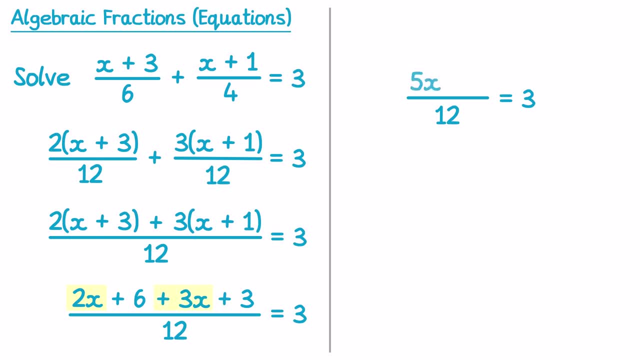 we've got 2x and 3x. that adds to make 5x, and then we've also got a 6, plus 3,, which gives you 9.. We've now turned this into a relatively straightforward equation to solve. We can multiply both sides by 12 to get rid of that fraction. If you multiply by 12 on the 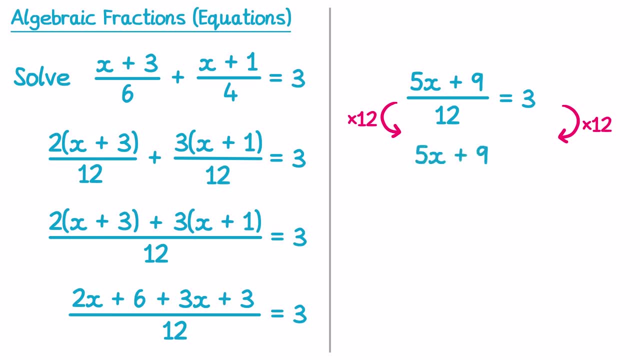 left, you get 5x plus 9, and if we multiply by 12 on the right, 3 times 12, is 36.. Then just subtract 9 from both sides, this will give you 5x equals 27,, and then divide both sides by 5, and this: 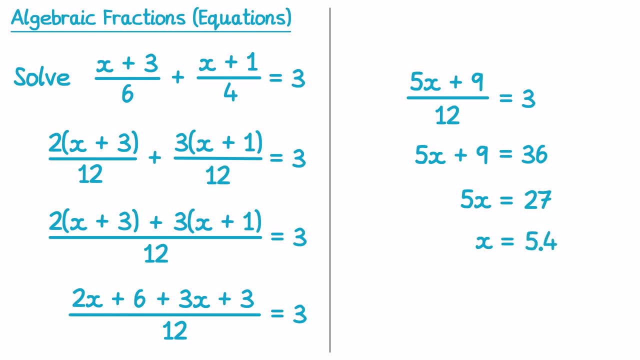 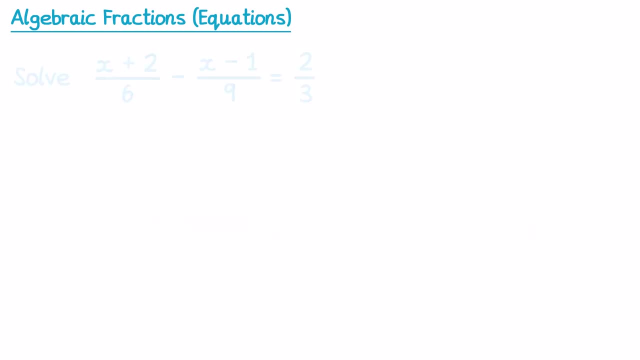 gives you: x equals 27 divided by 5, which is 5.4.. So the solution to this equation is 5.4.. Now let's try another example that's a bit more tricky, So for this one we're going to use the. 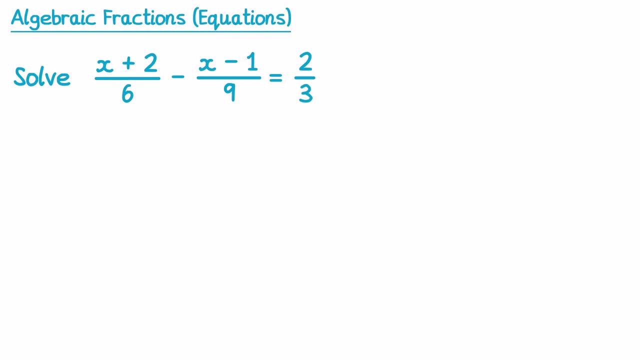 same approach. at first, we're going to leave the right hand side alone and try and combine the left hand side into one big fraction. Looking at my denominators this time of 6 and 9, the lowest common multiple is 18.. So I'm going to write both of these as something over 18.. 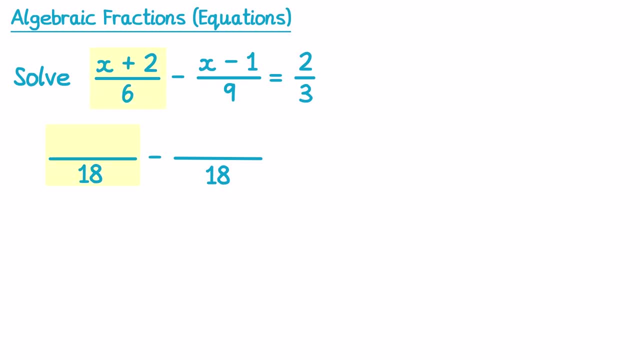 For the first fraction to get from 6 to 18, we multiply by 3, so we need to multiply x plus 2 on the top by 3 as well. so 3 lots of x plus 2.. For the second fraction to get from 6 to 18,: 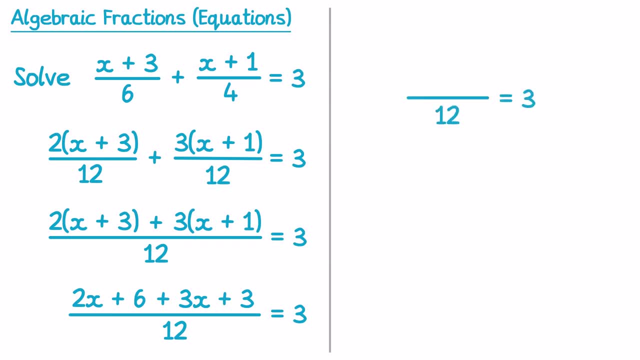 terms. So if we write the over 12 and equals 3,, we've got 2x and 3x. that adds to make 5x, and then we've also got a 6 and a plus 3, which gives you 9.. We've now 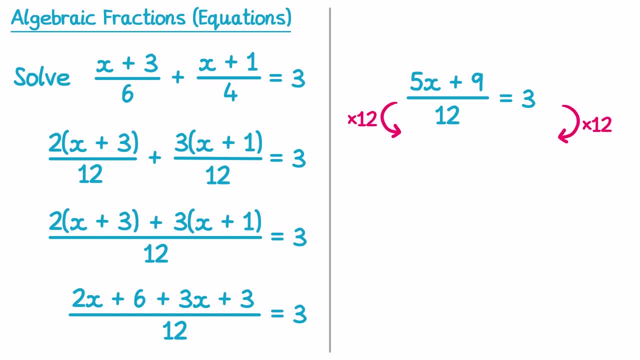 turned this into a relatively straightforward equation to solve. We can multiply both sides by 12 to get rid of that fraction. If you multiply by 12 on the left, you get 5x plus 9, and if we multiply by 12 on the right, 3 times 12. 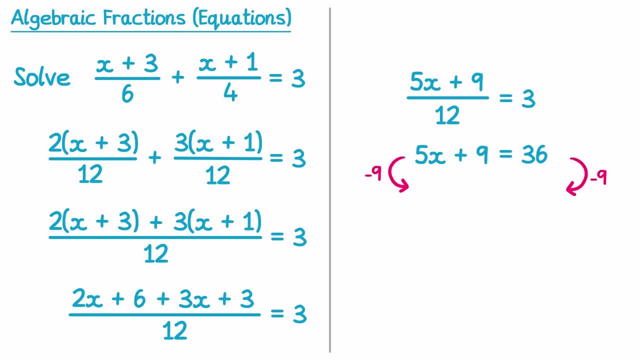 is 36.. Then just subtract 9 from both sides. this will give you 5x equals 27,. and then divide both sides by 5, and this gives you x equals 27 divided by 5, which is 5.9.. 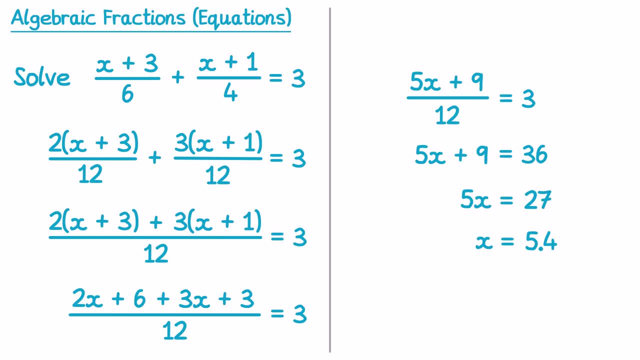 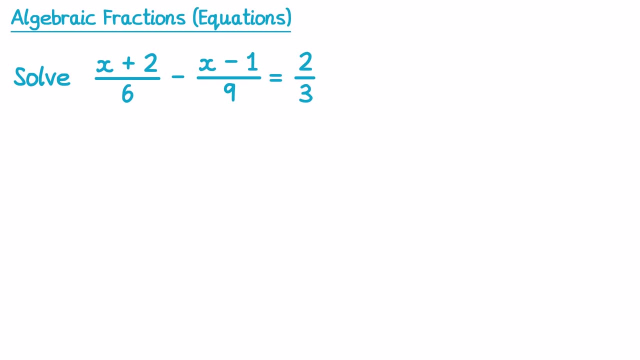 So the solution to this equation is 5.4.. Now let's try another example. that's a bit more tricky, So for this one we're going to use the same approach. at first we're going to leave the right hand side alone and try and combine the left hand. 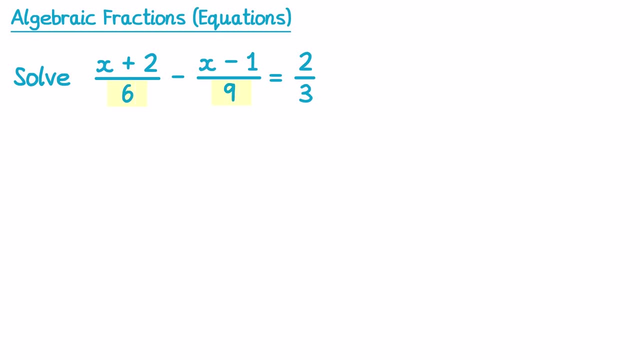 side into one big fraction. Looking at my denominators this time of 6 and 9, the lowest common multiple is 18, so I'm going to write both of these as something over 18.. For the first fraction to get from 6 to 18, we multiply by 3, so 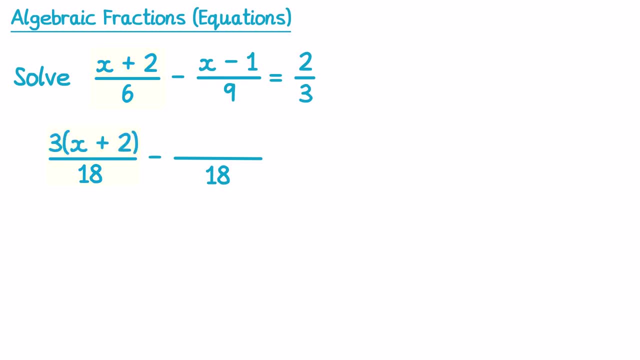 we need to multiply x plus 2 on the top by 3 as well, so 3 lots of x plus 2.. For the second fraction to get from 9 to 18, we multiply by 2, so we need 2 lots of the top. so 2 lots of x minus 1, and keep that right hand side, the. 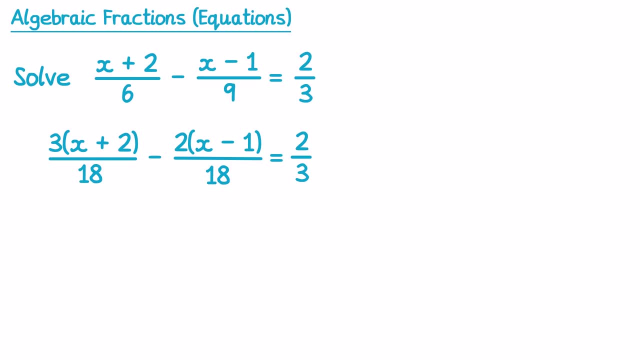 same equals 2 thirds. Now we have that common denominator, we can combine them into one big fraction, all over 18, so we have 3 lots of x plus 2, then in between them a subtraction sign, and then 2 lots of x minus 1, and keep that right hand side the same. that's 2 thirds. 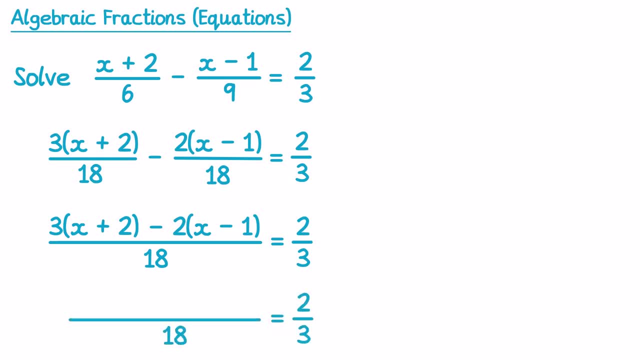 Then, as we did before, we're going to expand those brackets, so we'll write the over 18 and the 2 thirds down and then expand these brackets. We've got 3 lots of x, that's 3x 3. lots of positive: 2, that's plus 6.. Then we have negative 2 times x, that's negative. 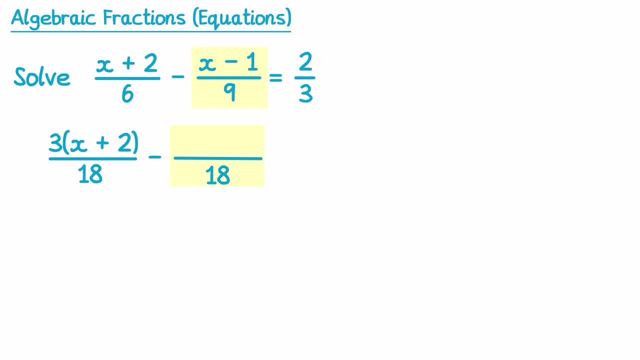 9 to 18. we multiply by 2, so we need 2 lots of the top, so 2 lots of x minus 1, and keep that right hand side. the same equals 2 thirds. Now we have that common denominator. we can combine them into. 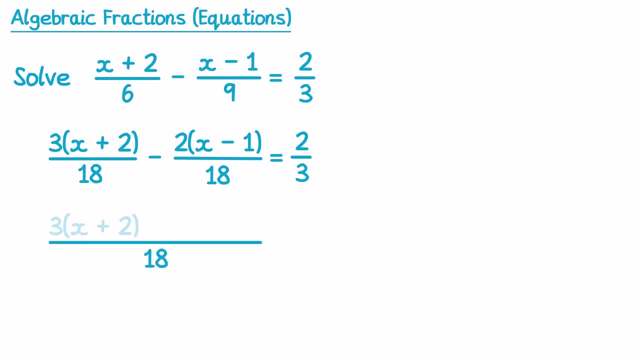 one big fraction all over 18. so we have 3 lots of x plus 2, then in between them a subtraction sign and then 2 lots of x minus 1 and keep that right hand side the same, that's 2 thirds. Then, as we did before, we're going to expand those brackets, so we'll write the over 18 and 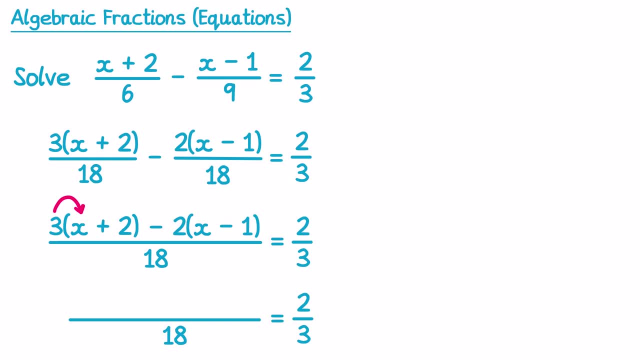 the 2 thirds down and then expand these brackets. we've got 3: lots of x, that's 3x. 3 lots of positive: 2, that's plus 6. then we have negative 2 times x, that's negative 2x. and you have to be really. 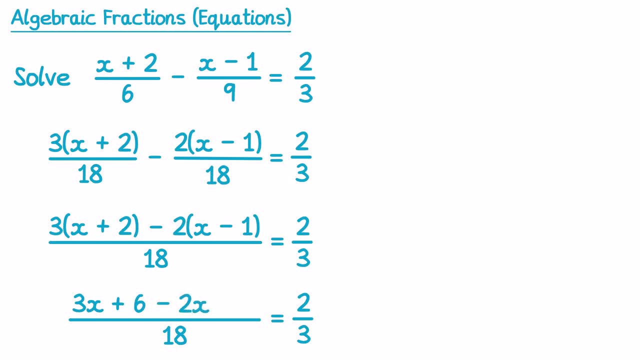 2x, and you have to be really careful on this one. this is a really common mistake. negative 2 times negative 1 is positive 2.. Then, as before, we'll collect the like terms on the numerator, so everything else can be written down as the same, and then on the top we've. 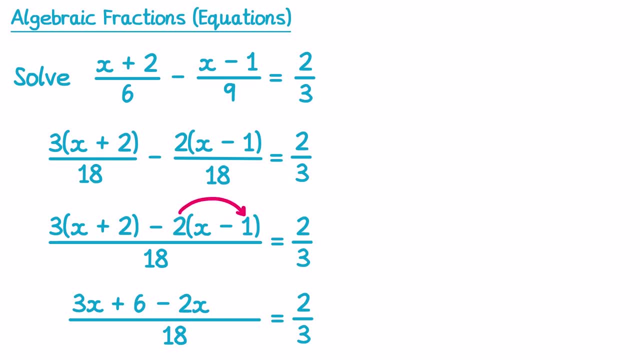 careful on this one. this is a really common mistake. negative 2 times negative 1 is positive 2.. Then, as before, we'll collect the like terms on the numerator so everything else can be written down as the same. and then on the top we've got 3x minus 2x. that's just 1x. and then we've got 6 plus 2. 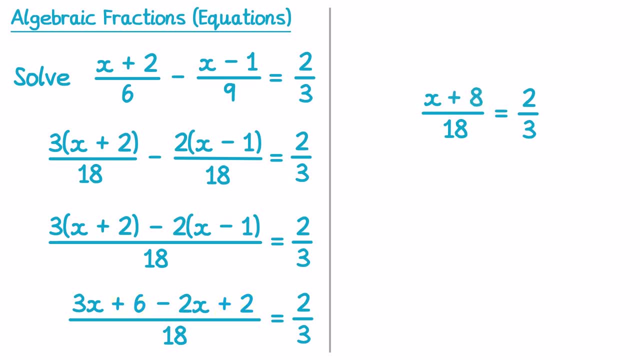 which is 8.. The next thing I would do here is multiply both sides by 18.. If we multiply by 18 on the left, that will cancel the 18 that's there. so we just have x plus 8. and if you multiply the right hand, 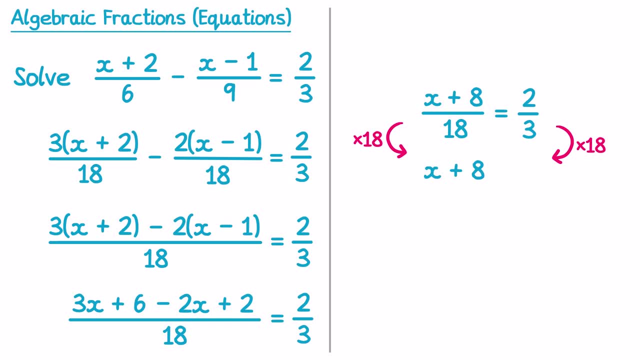 side by 18, we've got 2 thirds multiplied by 18. that's just the same as 2 thirds of 18.. 2 thirds of 18 is 12.. Finally, if we subtract 8 from both sides, we end up with the answer: x equals 4.. 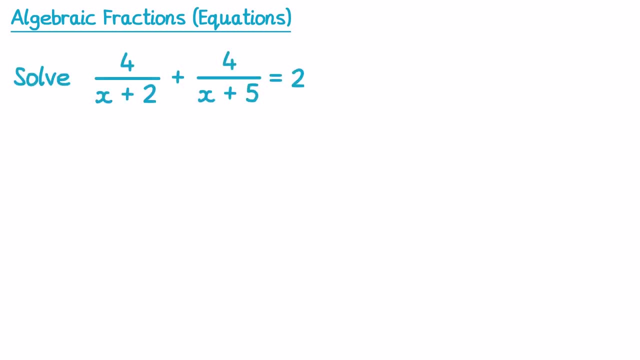 Now let's increase the difficulty once more and have a look at this question here. When we look at the denominators of these fractions, we can see they both have two terms. This means to find their lowest common multiple. we're going to need to multiply them together, So both of these fractions can be rewritten as something over x plus 2 x plus. 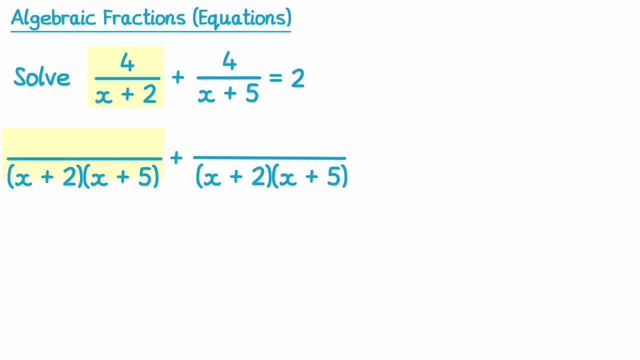 5.. Let's look at the left fraction first. so this one To get from x plus 2 to x plus 2 multiplied by x plus 5, we obviously multiply by x plus 5.. So we need to do this on the top as well. 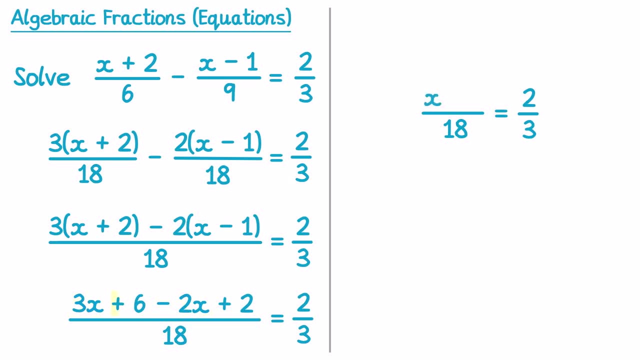 got 3x minus 2x, that's just 1x, and then we've got 6 plus 2,, which is 8.. The next thing I would do here is multiply both sides by 18.. If we multiply by 18 on the 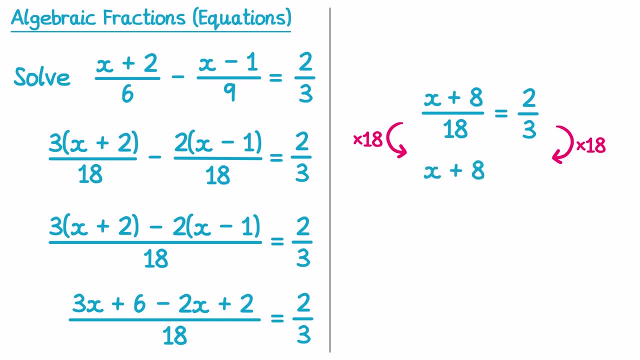 left. that'll cancel the 18 that's there. so we just have x plus 8.. And if you multiply the right hand side by 18, we've got 2 thirds multiplied by 18.. That's just the same as 2 thirds of 18.. 2 thirds of 18 is 12.. Finally, if we subtract 8 from both sides, we end up. 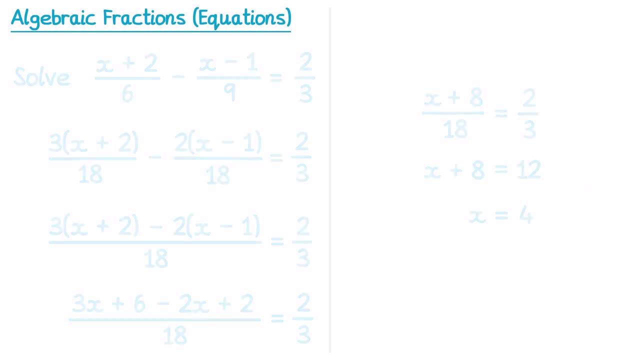 with the answer, x equals 4.. Now let's increase the difficulty once more and have a look at this question here. When we look at the denominators of these fractions, we can see they both have two terms. This means to find their lowest common multiple. 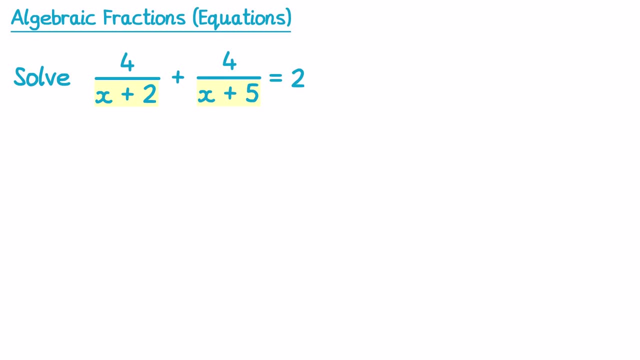 we're going to need to multiply them together, So both of these fractions can be rewritten as something over x plus 2, x plus 5.. Let's look at the left fraction first, so this one To get from x plus 2 to x plus 2 multiplied by x plus 5, we obviously multiply by x plus. 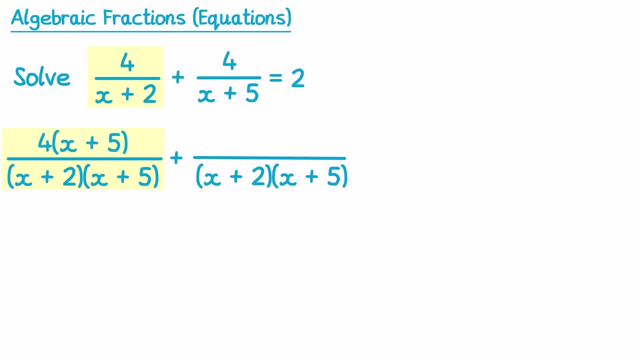 5.. So we need to do this on the top as well. so we need 4, lots of x plus 5.. And then we can look at the second fraction. So to get from x plus 5… to x plus 2, multiplied by x plus 5, we multiply by x plus 2.. So on the top we 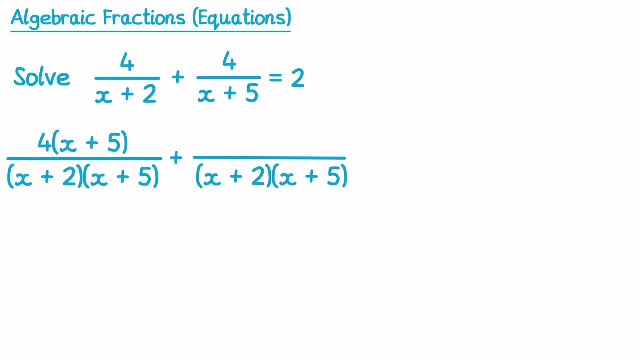 so we need 4, lots of x plus 5.. And then we can look at the second fraction. So to get from x plus 5 to x plus 2 multiplied by x plus 5, we multiply by x plus 2.. So on the top we need to multiply by x. 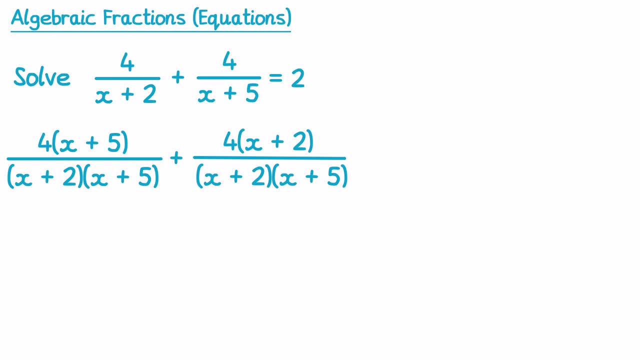 plus 2 as well, and that's 4 lots of x plus 2.. And of course, the right hand side is still just 2.. Now that we have this common denominator, we can write them as one big fraction all over: x plus 2 x. 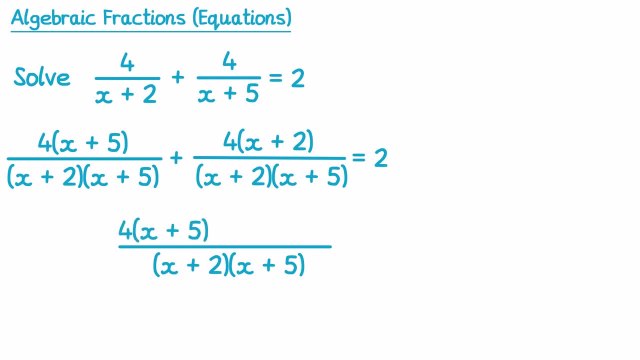 plus 5.. So on the numerators we have 4 lots of x plus 5, then in between them we have a plus sign and then 4 lots of x plus 2, and the right hand side is still equals 2.. We can now do some expanding and then simplifying. 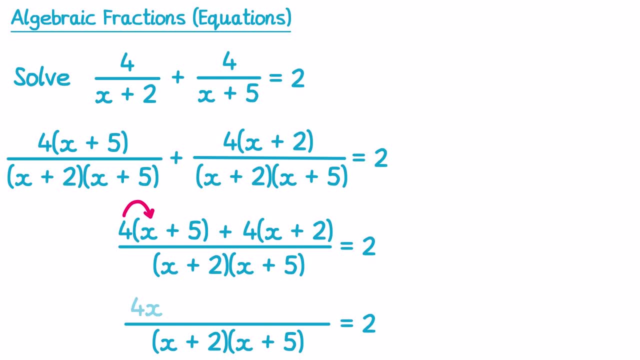 So if we expand out the numerator, we've got 4 times x, which is 4x, 4 times 5, which is plus 20, 4 times x, which is 4x again, and then 4 times 2, that's a positive 8.. 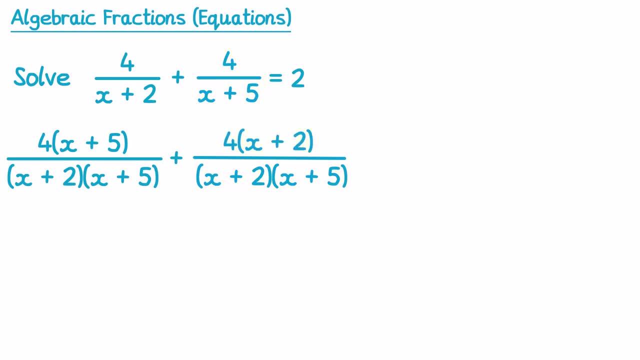 need to multiply by x plus 2 as well, and that's 4, lots of x plus 2.. And of course, the right-hand side is still just 2.. Now that we have this common denominator, we can write them as one big fraction all over: x plus 2, x plus 5.. So on the 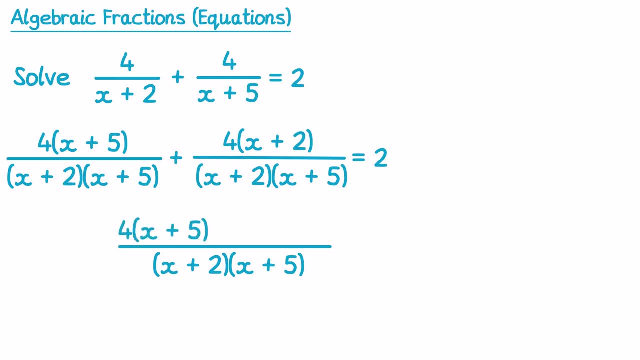 numerators. we have 4 lots of x plus 5, then in between them we have a plus sign and then 4 lots of x plus 2, and the right-hand side is still equals 2.. We can now do some expanding and then simplifying. So if we expand out the 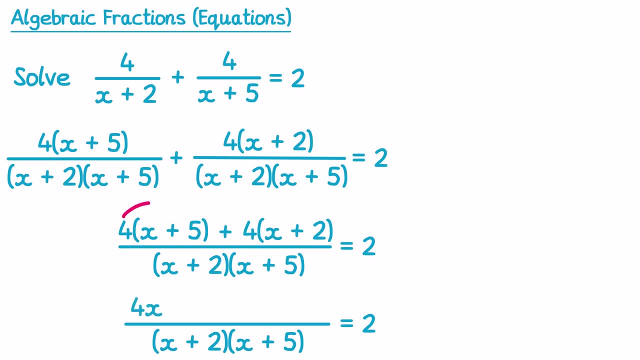 numerator. we've got 4 times x, which is 4x, 4 times 5, which is plus 20,, 4 times x, which is 4x again, and then 4 times 2, that's a positive 8.. Next we need to do: 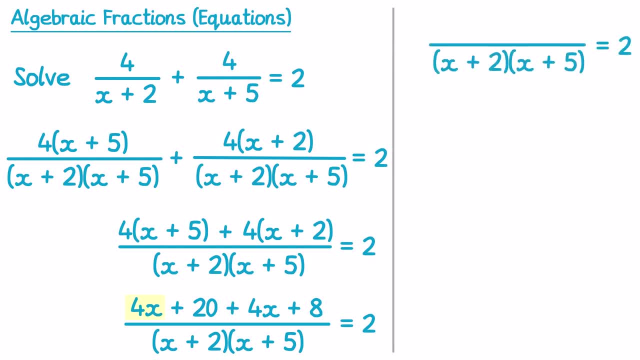 the simplifying of the numerator. So on the top here we have 4x plus 4x, which is 8x, and then we also have 20 plus 8, which is 28.. Next we're going to multiply both sides of this equation by both numbers. 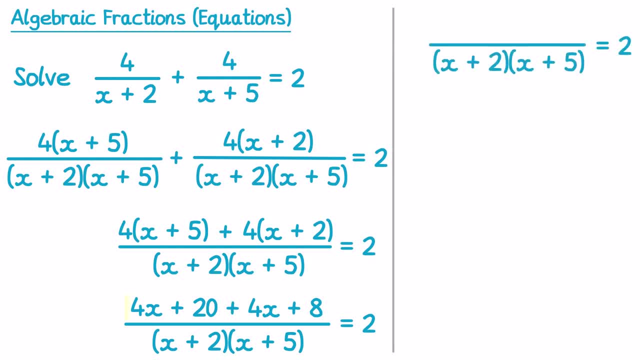 Next we need to do the simplifying of the numerator. So on the top here we have 4x plus 4x, which is 8x, and then we also have 20 plus 8, which is 28.. Next we're going to multiply both sides of this equation by both of those brackets. 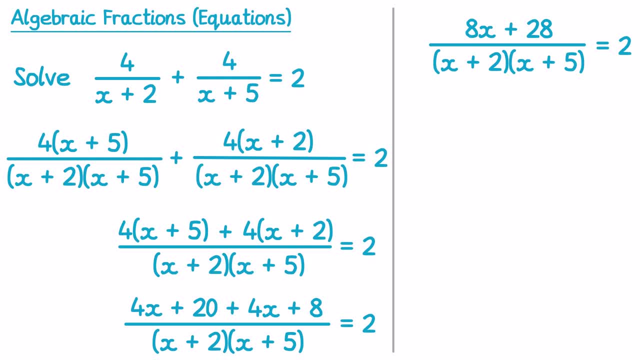 that are on that denominator, So by x plus 2 and x plus 5.. This will clear the fraction on the left hand side to give us 8x plus 28,. but on the right hand side we'll have 2 lots of x plus 2, x plus 5.. 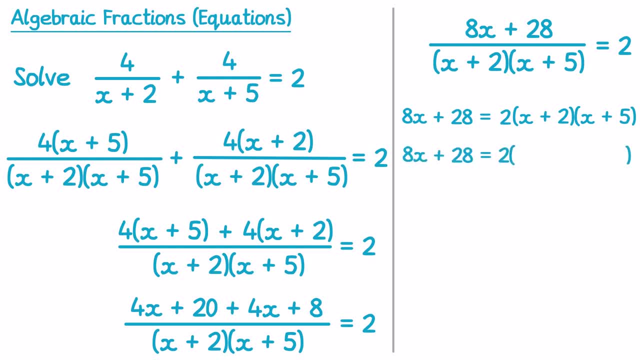 Next we'll leave the left hand side alone and then we've got 2 lots and then we'll expand those brackets and whatever we get will go inside this much larger bracket here. So if we expanded that double bracket we'd have x times x, that's x squared. we then 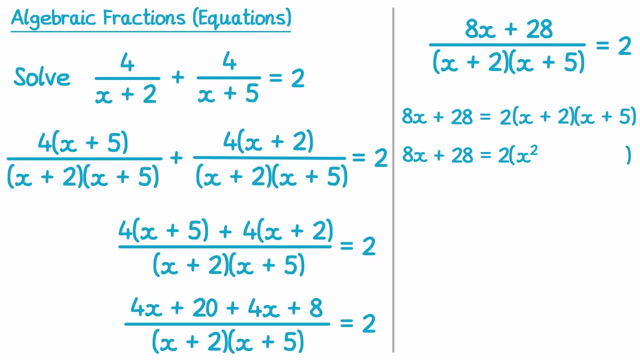 have x times 5, which is 5x, and 2 times x, which is 2x and 5x, and 2x adds to make 7x, And then, finally, we'd have 2 times 5, which is 10.. 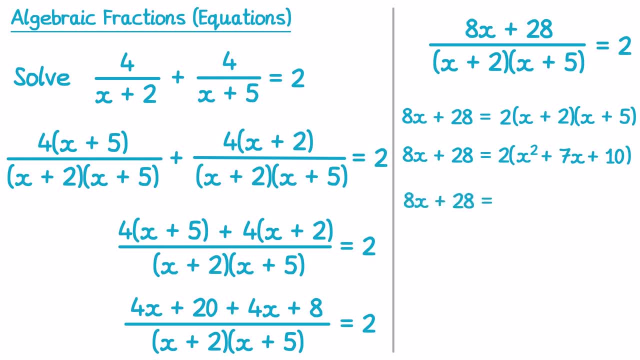 On the right hand side. we can then expand this bracket. so if we leave the left hand side alone, on the right hand side we have 2 lots of everything that's in that bracket. So 2 lots of x squared, 2 lots of 7x, that's 14x. 2 lots of 10, that's 20.. 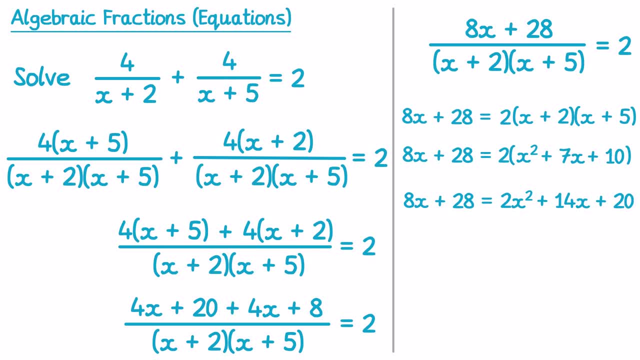 You can now see we have a quadratic equation to solve. When we solve these, we need to set one of the sides equal to 0.. Since the 2x squared is on the right hand side, I'm going to make the left hand side. 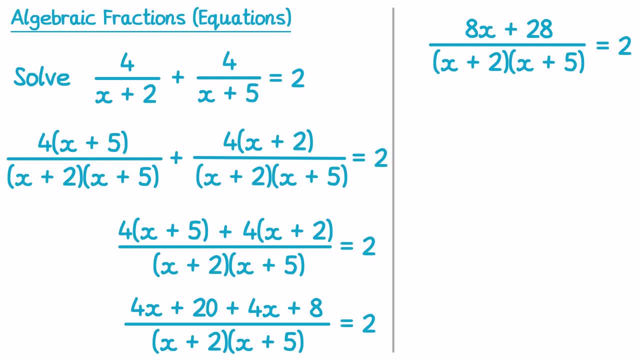 those brackets that are on that denominator, so by x plus 2 and x plus 5.. This will clear the fraction on the left hand side to give us 8x plus 28,. but on the right hand side we'll have two lots of x plus 2, x plus 5.. Next we'll leave the left hand side alone, and then we've got two. 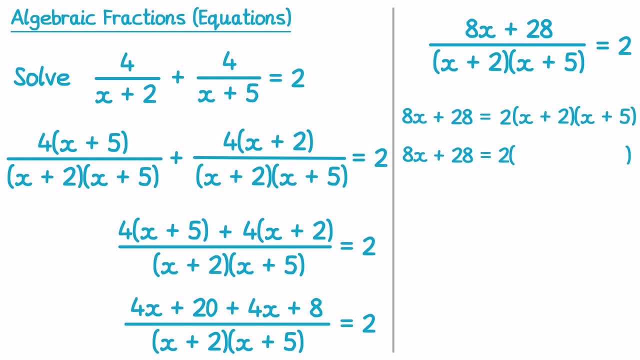 lots, and then we'll expand those brackets and whatever we get will go inside this much larger bracket here. So if we expanded that double bracket we'd have x times x, that's x squared. we then have x times 5, which is 5x, and 2 times x, which is 2x and 5x, and 2x adds to make 7x. 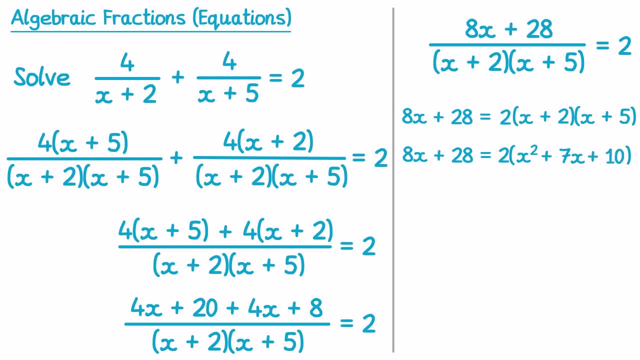 and then finally we'd have 2 times 5, which is 10.. On the right hand side we can then expand this bracket. so if we leave the left hand side alone, on the right hand side we have two lots of everything that's in that bracket. So two lots of x squared, two lots of 7x, that's 14x. two lots of. 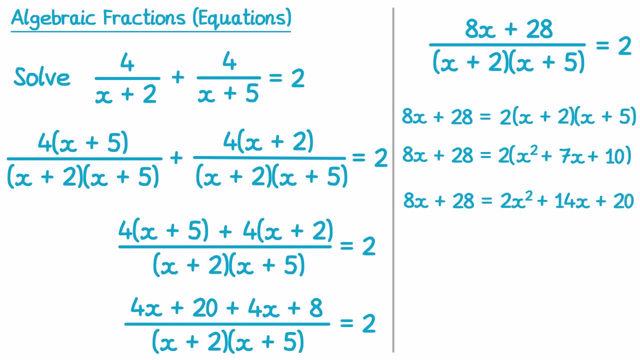 10, that's 20.. You can now see we have a quadratic equation to solve. When we solve these, we need to set one of the sides of the equation to be equal to one of the sides of the equation to be equal to zero. Since the 2x squared is on the right hand side, I'm going to make the left hand side equal. 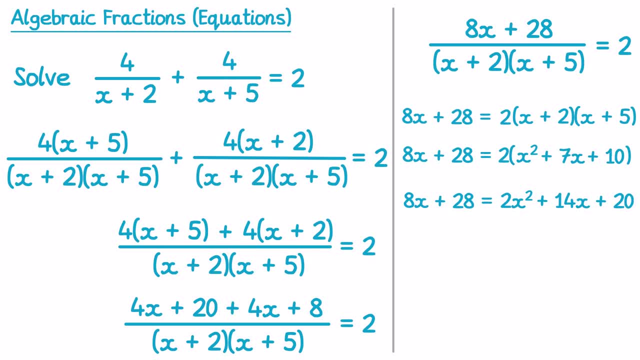 to zero. To do this I need to take away 8x and also take away 28 from both sides. If I took away those from the left hand side, I'd get zero, and if I take those away from the right hand side, the 2x. 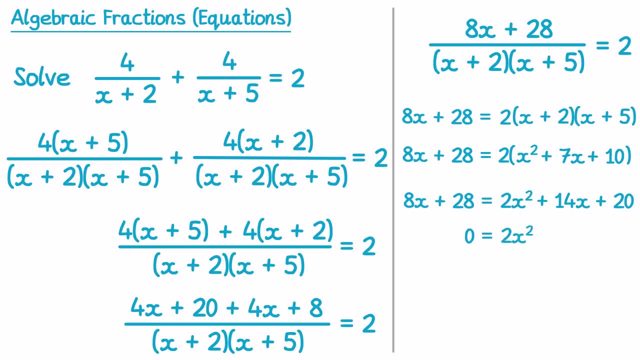 squared will remain unchanged. but then I need to take the 8x away from the 14x, which is 6x, and then take the 28 away from the 20, which is negative 8.. Now there's a common factor of 2 here to all terms, so I can divide both sides by 2.. 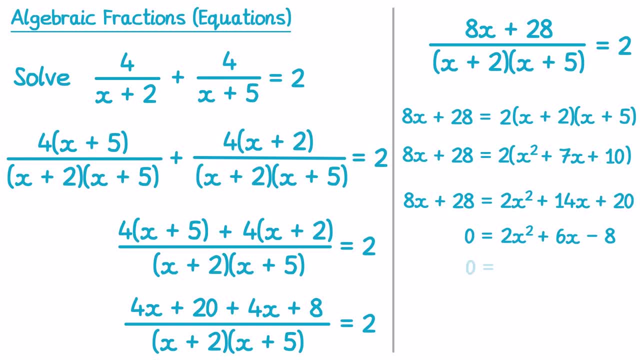 If I divide the left hand side by 2,, 0 divided by 2 is still 0. but then on the right hand side, 2x squared divided by 2 is 1x squared, 6x divided by 2 is 3x and negative. 8 divided by 2 is negative. 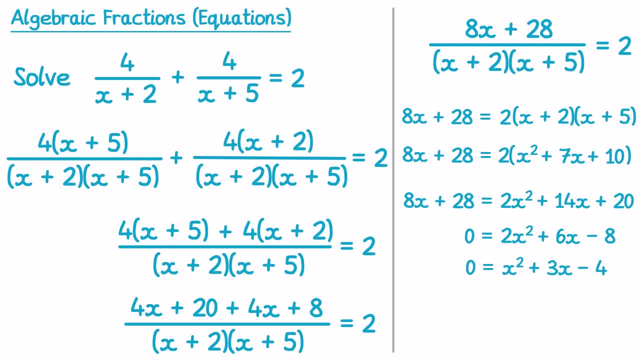 4.. Fortunately for us, this quadratic will factorise, so on the left hand side we have 0, and the right hand side will factorise to give x plus 4, x minus 1.. This leads us to two solutions. either the first bracket is 0, so x plus 4 equals 0, in which case x is negative 4, or the second bracket. 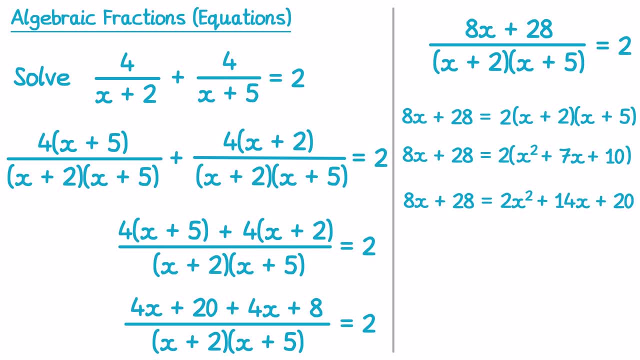 equal to 0.. To do this, I need to take away 8x and also take away 28 from both sides. If I took away those from the left hand side, I'd get 0, and if I take those away from the right hand side, the 2x squared will remain unchanged. but then I need to take the 8x. 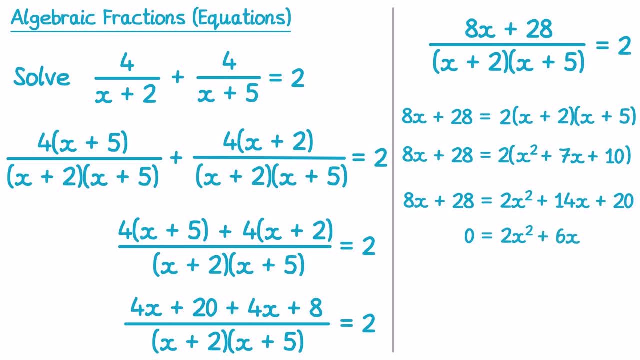 away from the 14x, which is 6x, and then take the 28 away from the 20, which is negative 8.. Now there's a common factor of 2 here, to all terms, so I can divide both sides by 2.. 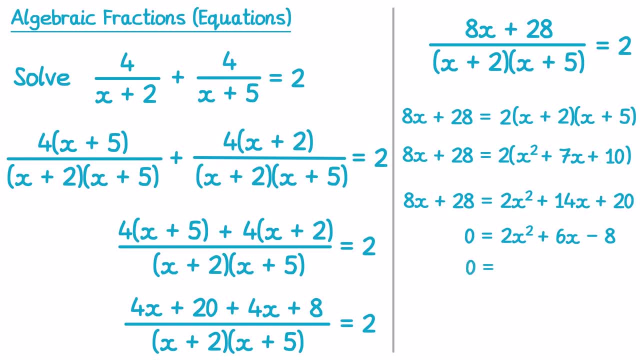 If I divide the left hand side by 2,, 0 divided by 2 is still 0. But then on the right hand side, 2x squared divided by 2 is 1x squared, 6x divided by 2. 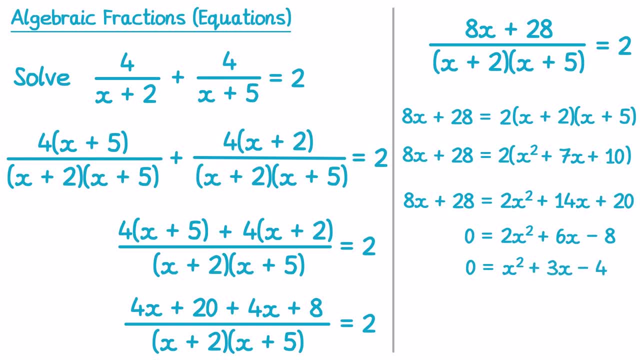 is 3x and negative 8 divided by 2 is negative 4.. Fortunately for us, this quadratic will factorise, so on the left hand side we have 0, and the right hand side will factorise to give x plus 4, x minus 1.. 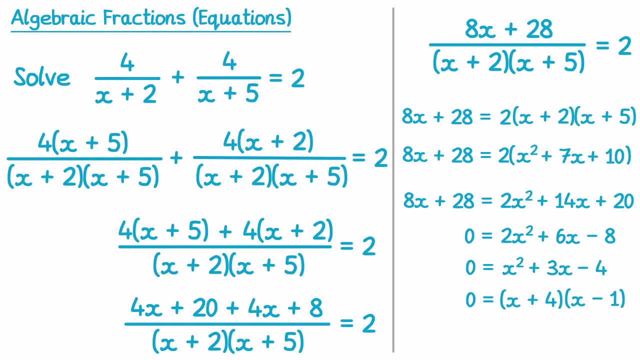 This leads us to two solutions. either the first bracket is 0,, so x plus 4 equals 0,, in which case x is negative 4, or the second bracket equals 0,, so x minus 1 equals 0, gives: 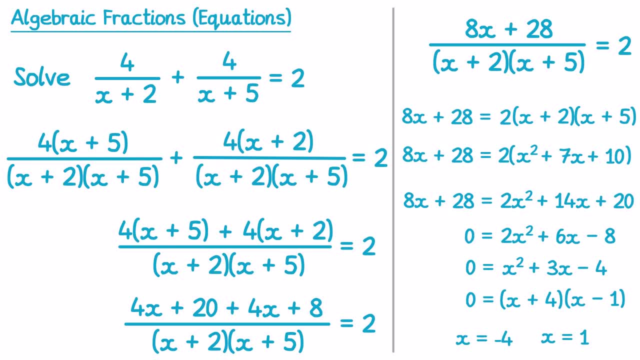 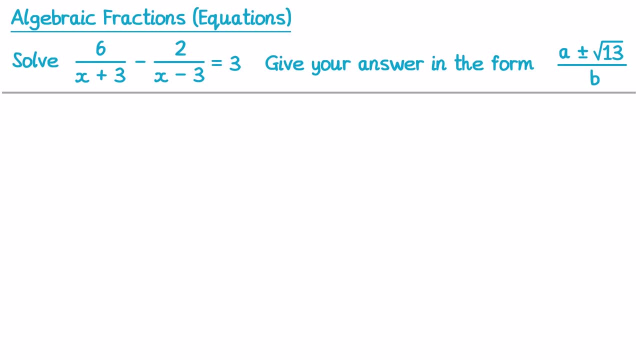 us, the solution x equals positive 1.. Now let's have a look at an even trickier question. So for this one we need to solve an equation, but we've told we need to give the answer in a particular form: a plus or minus square root, 13 over b. 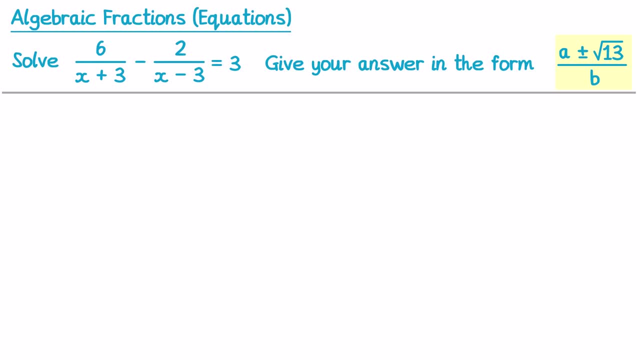 This is a clear indication that when we get to a quadratic, at the end it's not going to factorise anymore. We either need to use the quadratic formula or complete the square to get the solutions. So let's go ahead and try and solve this one. 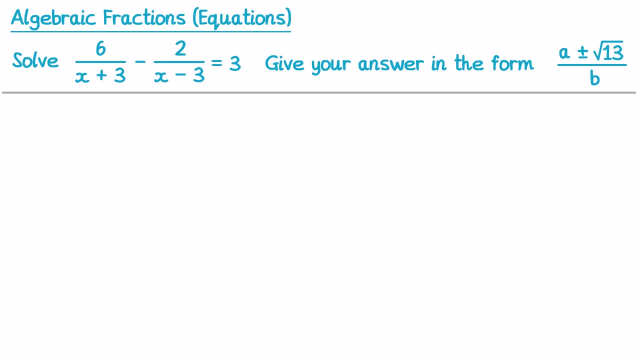 So first of all we'll look at those denominators and we can see we've got x plus 3, x minus 3.. These will become our denominators. Then we compare the first fractions so to get from x plus 3 to x plus 3, x minus 3,. 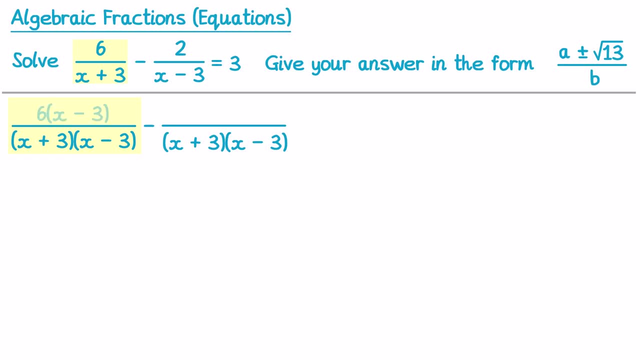 we multiply by x minus 3, so we need to multiply that 6 on the top by x minus 3.. And when we compare the second fractions, this time we've multiplied by x plus 3, so on the top we need 2, lots of x plus 3.. 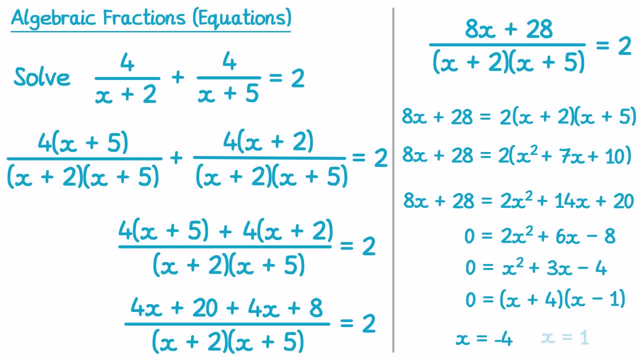 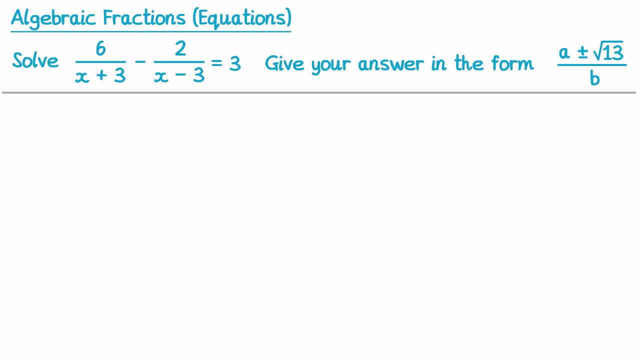 is 0. so x minus 1 equals 0 gives us the solution: x equals positive 1.. Now let's have a look at an even trickier question. So for this one we need to solve an equation, but we've told we need to give the answer in a particular form: a plus or minus square root 13. 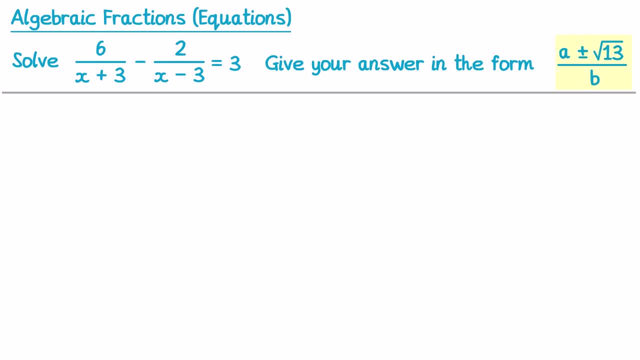 over b. This is a clear indication that when we get to a quadratic, at the end it's not going to factorise anymore. We either need to use the quadratic formula or complete the square to get the solutions. So let's go ahead and try and solve this one. 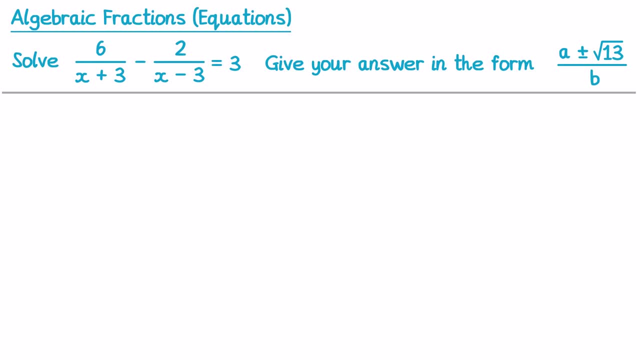 First of all we'll look at those denominators and we can see we've got x plus 3, x minus 3, so the product of those will become our denominators. Then we compare the first fractions. so to get from x plus 3 to x plus 3, x minus 3, we multiply by x minus 3, so we need. 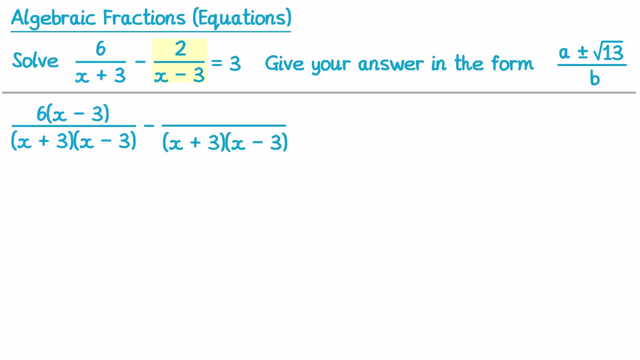 to multiply that 6 on the top by x minus 3, and when we compare the second fractions, this time we've multiplied by x plus 3, so on the top we need two lots of x plus 3 and this equals 3.. Now we can combine them into one big fraction over that common denominator. 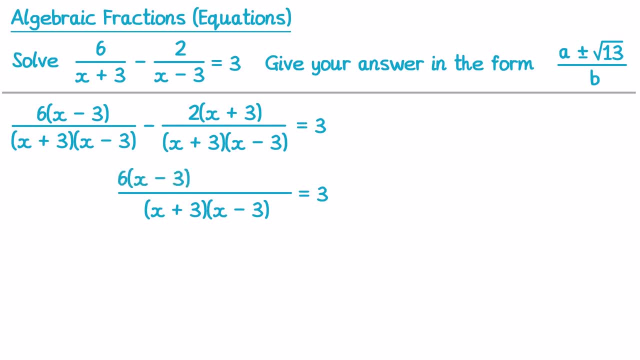 we have 6 lots of x minus 3- in between the fractions is the subtraction sign- and then 2 lots of x plus 3.. Now we can expand out those brackets. so on the top we've got 6 times x, that's 6x, 6 times negative, 3 negative 18, negative 2 times x, negative 2x and a negative 2 multiplied. 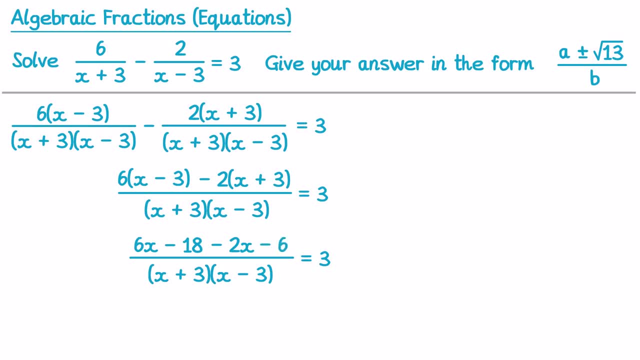 by a positive 3, that's a negative 6. Then we can collect those like terms. so on the top, we've got 6x: take 2x, that's 4x. and we've got 6x, take 2x, that's 4x. and we've got 6x: take 2x, that's 4x. 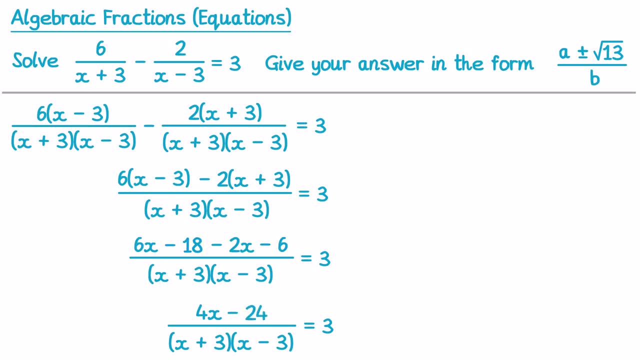 and then negative 18. subtract 6, that's negative 24.. Then we would multiply both sides by that denominator: x plus 3, x minus 3.. This will clear the fraction on the left hand side. so you've just got 4x minus 24, but on the right hand side we have 3- lots of x plus 3, x minus 3.. To solve this we'll 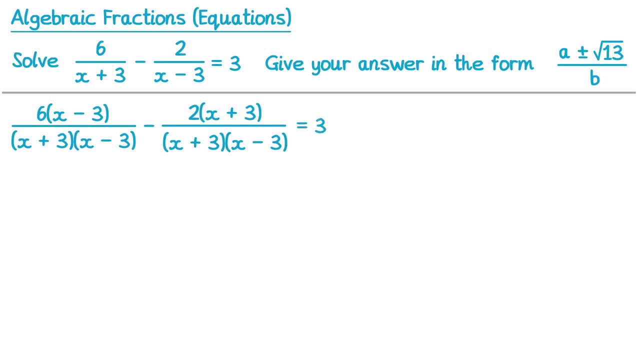 And this equals 3.. Now we can combine them into one big fraction over that common denominator. We have 6 lots of x minus 3.. In between the fractions is a square root 13 over b, That's a subtraction sign, And then 2 lots of x plus 3.. 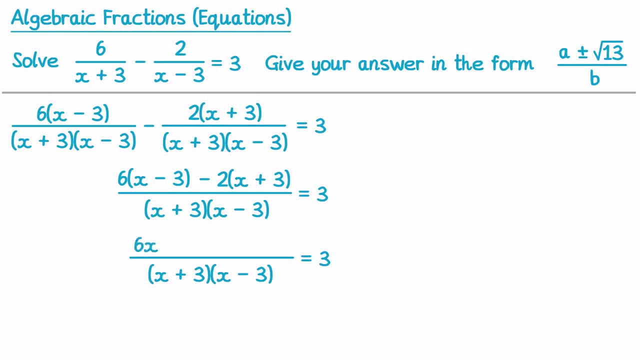 Now we can expand out those brackets. so on the top we've got 6 times x, that's 6x, 6 times negative, 3, negative 18, negative 2 times x, negative 2x and a negative 2 multiplied. 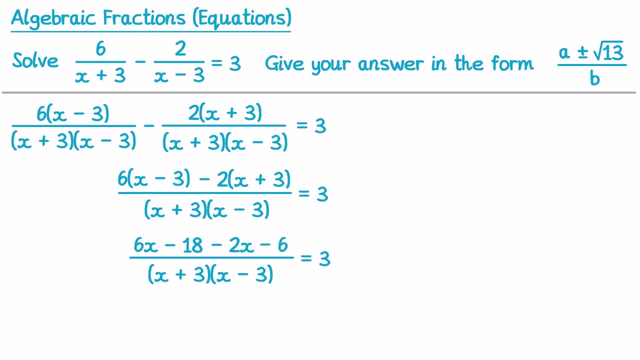 by a positive 3, that's a negative 6. Then we can collect those like terms. so on the top we've got 6x. take 2x, that's 4x, and then negative 18, subtract 6,, that's negative 24.. 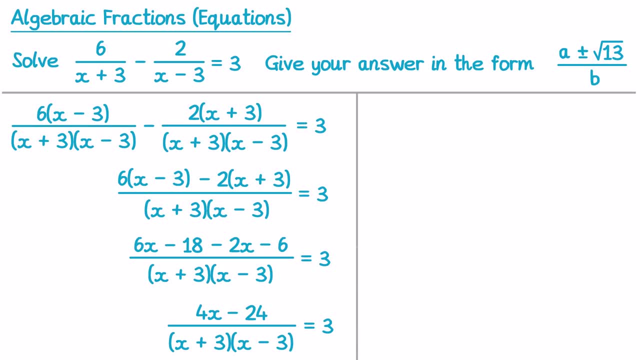 Then we would multiply both sides by that denominator: x plus 3, x minus 3.. This will clear the fraction on the left hand side. so you've just got 4x minus 24, but on the right hand side we have 3 lots of x plus 3, x minus 3.. 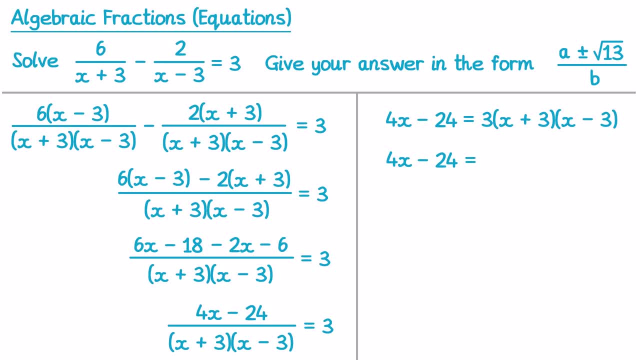 To solve this, we'll leave the left hand side alone and on the right hand side we've got 3- lots of whatever we get when we expand these two brackets. Well, this one's the difference of two squares: If we do x times x, we get x squared, and then we have x times negative, 3 negative, 3x. but 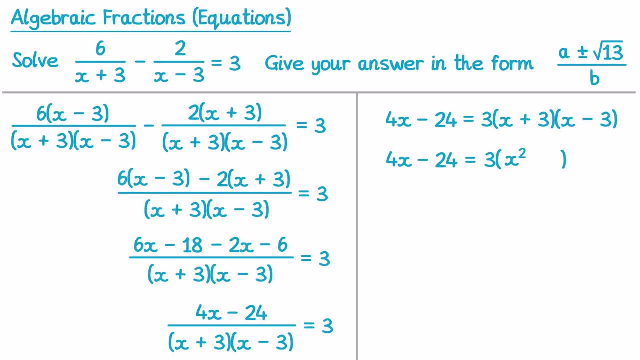 also positive 3 times x, which is positive 3x. So those x terms will cancel. and then we have 3 times negative 3, which is negative 9. So we have 4x minus 24, and then, if we expand this bracket 3, lots of x squared is 3x squared. 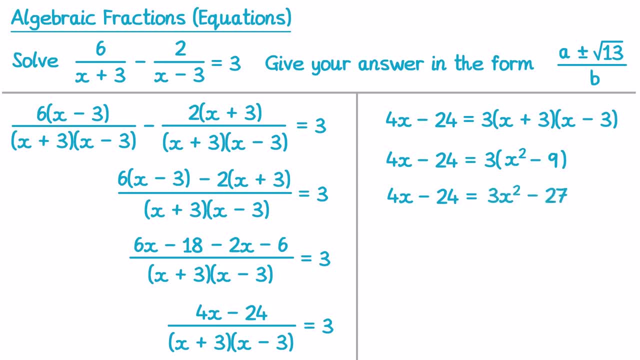 and 3, lots of negative. 9 is negative 27.. So you can see, we do have a quadratic and we need to get one of the sides to be equal to 0.. Once again, I'm going to make that the left hand side. 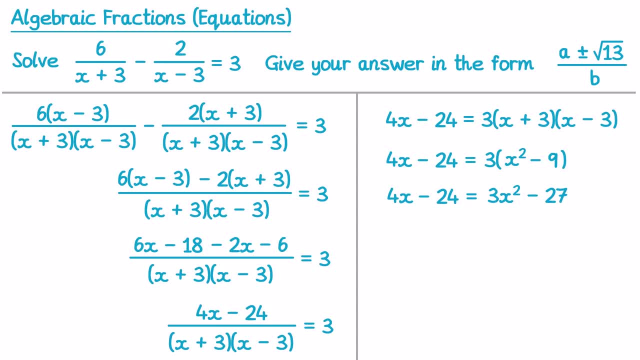 So to make the left hand side equal to 0, I would need to subtract 4x and then add 24 to both sides. So if I do that, on the left I get 0, of course, And on the right hand side I get 3x squared. that remains unchanged. 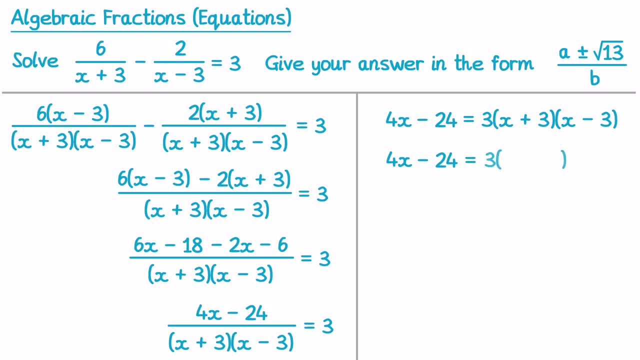 leave the left hand side alone, and on the right hand side we've got 3, lots of whatever we get when we expand these two brackets. Well, this one's the difference of two squares. if we do x times x, we get x squared, and then we have x times negative, 3 negative 3x, but also positive 3 times x, which is: 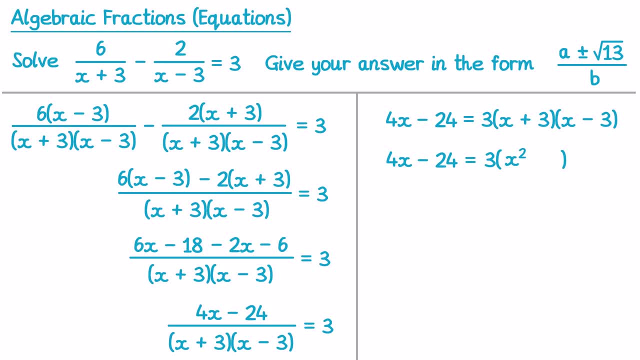 positive 3x, so those x terms will cancel. and then we have 3 times negative 3, which is negative 9. So we have 4x minus 24 and then, if we expand this bracket 3, lots of x squared is 3x squared. 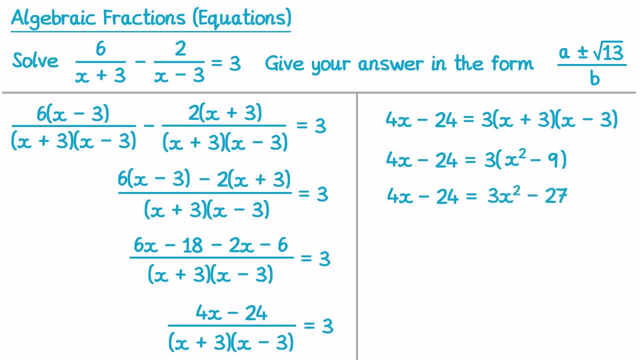 and 3, lots of negative. 9 is negative 27.. So you can see, we do have a quadratic and we need to get one of the sides to be equal to 0. Once again, I'm going to make that the left hand side, So to 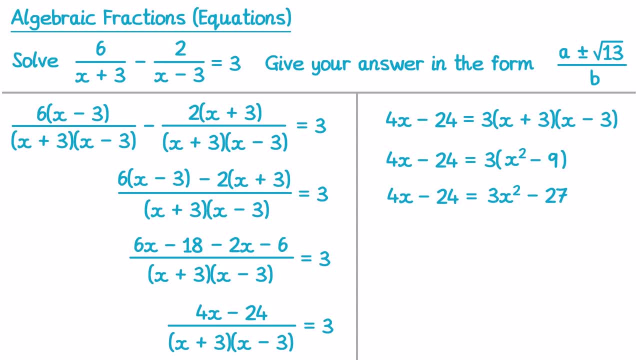 make the left hand side equal to 0, I would need to subtract 4x and then add 24 to both sides. So if I do that, on the left I get 0, of course, and on the right hand side I get 3x squared. 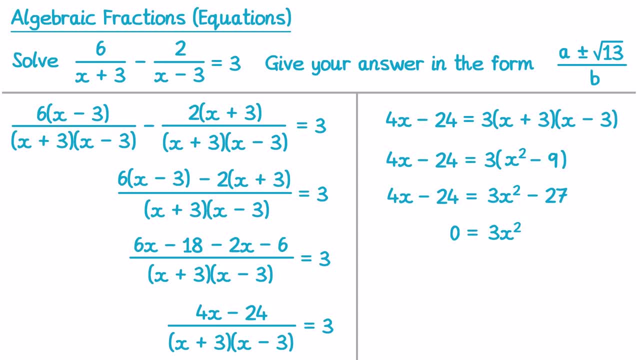 that remains unchanged. then I subtracted 4x and there's no x term there already, so that's just negative 4x. and then we need to add 24 to negative 27, which gives us negative 3.. So we end up with this quadratic equation here to solve. Now, remember, we know from the form they 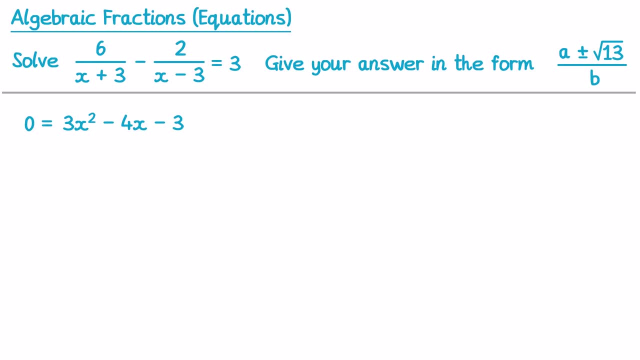 want the answer in. we need to solve this using the formula or completing the equation, And this one's probably going to be much easier using the quadratic formula. So we need to find the values of a, b and c. they're the coefficients of x squared. 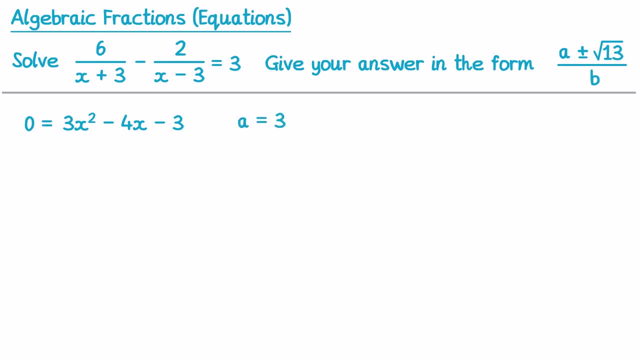 x and the constant term. So the coefficient of x squared is 3, the coefficient of x is negative 4 and the constant term at the end is negative 3.. So a is 3, b is negative 4 and c is negative 3.. Now we can substitute those values into the. 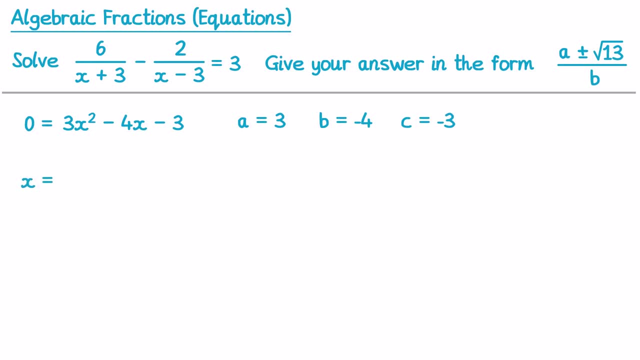 quadratic formula It's x equals negative b. well, b is already negative, so if we did negative b it would become positive. so it's actually a positive 4 plus or minus the square root of then b squared. so negative 4 squared subtract 4, lots of a, which is 3, multiplied by c, which is 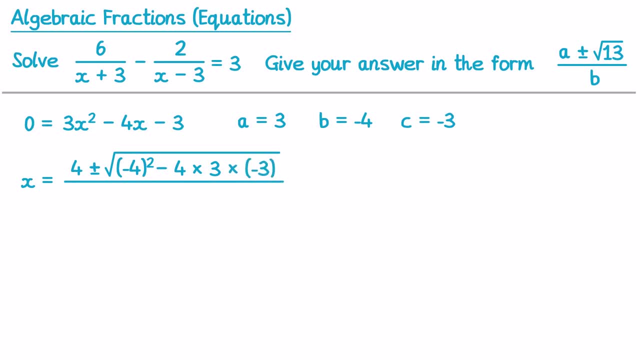 negative 3, and all of this is divided by 2 lots of a, and 2 lots of a is 2 lots of 3, so 6.. Now this question would actually be a non-calculator question, so we're going to need to work out the value of the number that's inside that square root. So let's write: x equals. 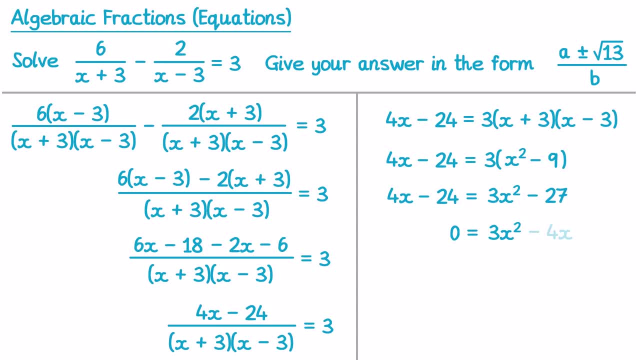 Then I subtracted 4x and there's no x term there already, so that's just negative 4x. And then we need to add 24 to negative 27, which gives us negative 3.. So we end up with this quadratic equation here to solve. 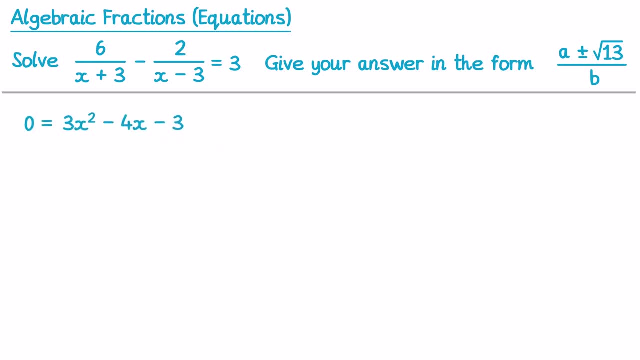 Now remember, we know from the form they want the answer in. we need to solve this using the formula or completing the square, and this one's probably going to be much easier using the quadratic formula. So we need to find the values of a, b and c. 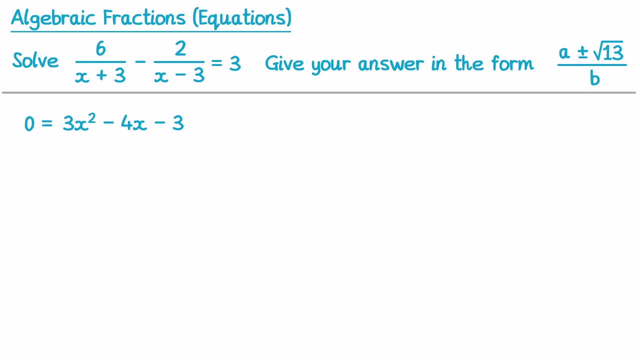 They're the coefficients of x squared. That's all x and the constant term. So the coefficient of x squared is 3, the coefficient of x is negative 4 and the constant term at the end is negative 3.. So a is 3, b is negative 4 and c is negative 3.. Now we can substitute those. 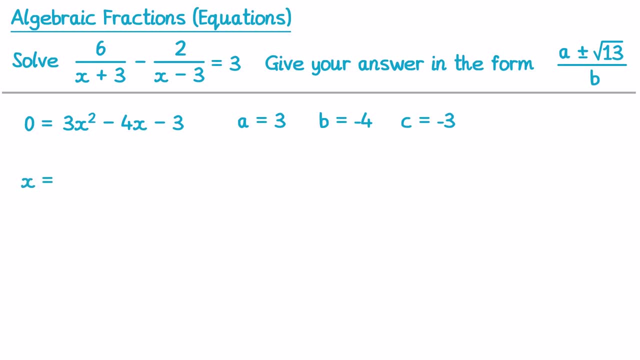 values into the quadratic formula. It's: x equals negative b. well, b is already negative, so if we did negative b it will become positive. so it's actually a positive 4, plus or minus the square root of then b squared, so negative 4. 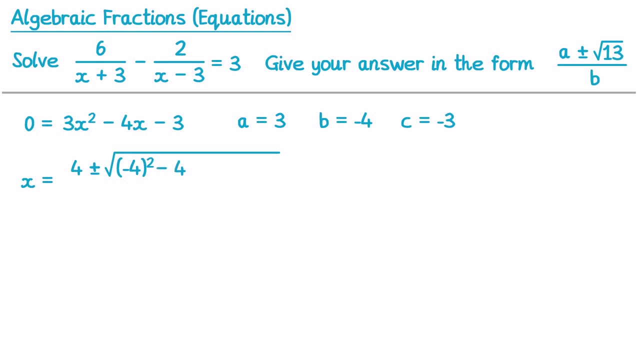 squared, subtract 4 lots of a, which is 3, multiplied by c, which is negative 3, and all of this is divided by 2 lots of a, and 2 lots of a is 2 lots of 3, so 6.. Now, this question would actually be a non calculator question, so we're going to 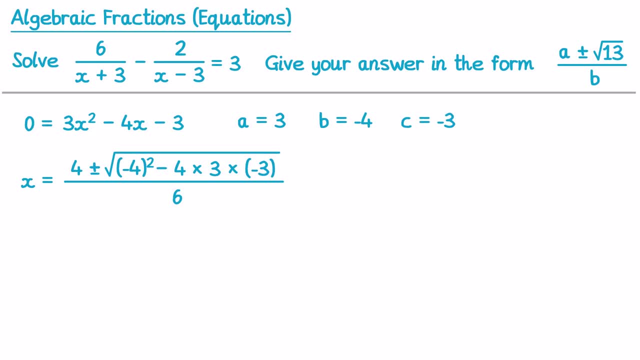 need to work out the value of the number that's inside that square root. So let's write: x equals 4 plus or minus the square root of over 6, but we'll work out what's inside that square root. So if we did negative 4 squared, that would be negative 4 multiplied by. 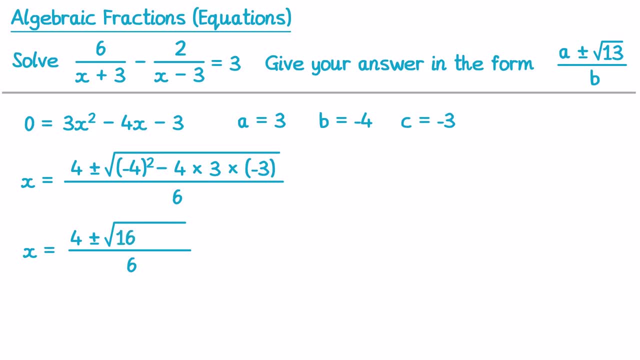 itself, so 16, and then, if we did negative 4, multiplied by 3, that's negative 12, and then multiply that by negative 3, that becomes a positive 36. So we end up with 16 plus 36 inside that square root. You can add those two together, that's 52. so 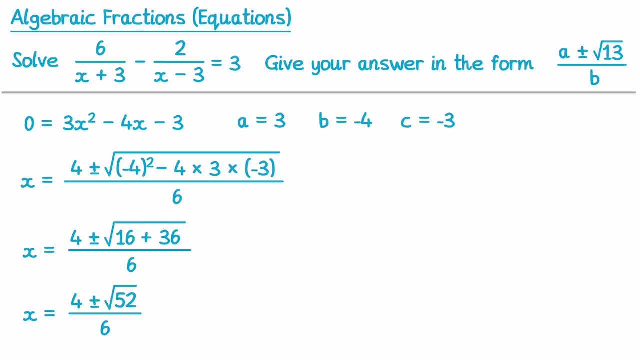 x equals 4 plus or minus square root 52 over 6.. Next, what we need to do is simplify that square root. So, using our third rules, if we take root 52, that could be expressed as root 4 multiplied by root 13.. The square root 4 is just 2, so this is 2 root 13.. So in 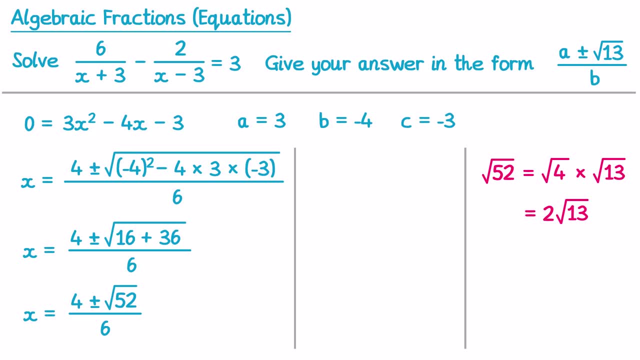 place of root 52 we could write 2 root 13, so it's x equals 4 plus or minus 2 root 13, now over 6.. Now this is looking a lot like the answer, but we're still not quite there. That one just has one square root 13 and we have 2.. The reason for? 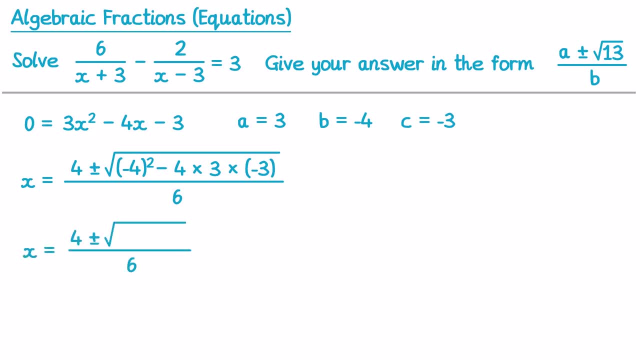 4 plus or minus the square root of over 6, but we'll work out what's inside that square root. So if we did negative 4 squared, that would be negative 4 multiplied by itself, so 16. and then if we did negative 4 multiplied by 3, that's negative 12, and then multiply that by 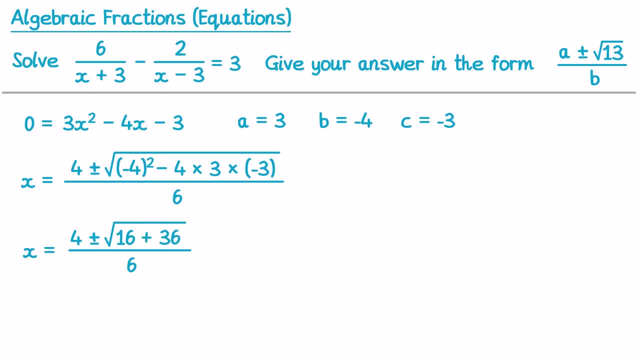 negative 3, that becomes a positive 36.. So we end up with 16 plus 36 inside that square root. You can add those two together, that's 52. so x equals 4 plus or minus square root, 52 over 6.. 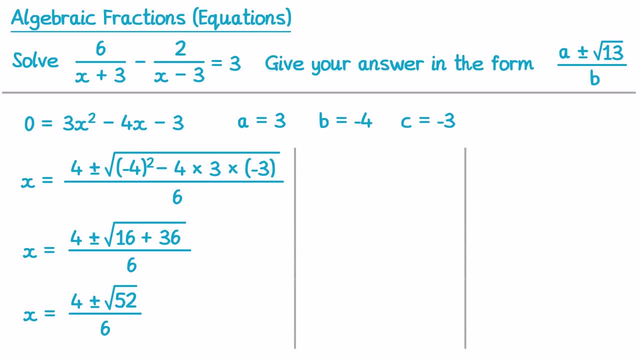 Next, what we need to do is simplify that square root 52.. So, using our assert rules, if we take root 52, that could be expressed as root 4 multiplied by root 13.. The square root 4 is just 2, so this is 2 root 13.. So in place of root 52 we could write 2 root 13, so it's x equals 4 plus or minus. 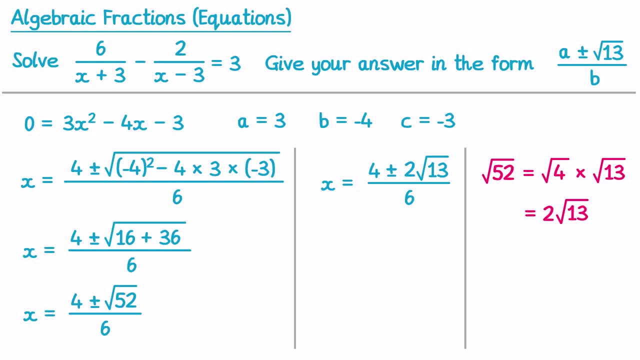 2 root 13, now over 6.. Now this is looking a lot like the answer, but we're still not quite there, that one just has one square root 13 and we have two. The reason for that is we have a common fact for a 2 here: If we divide all terms by 2, we get x equals. If we divide the 4 by 2, we get 2.. 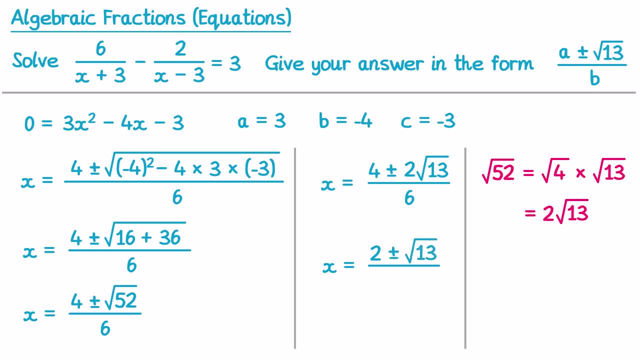 Divide 2 root 13 by 2, you get 1 root 13, and divide 6 by 2, you get 3.. This answer now matches the form we were asked in the question. You can see the value of a is 2 and the value of b is 3.. 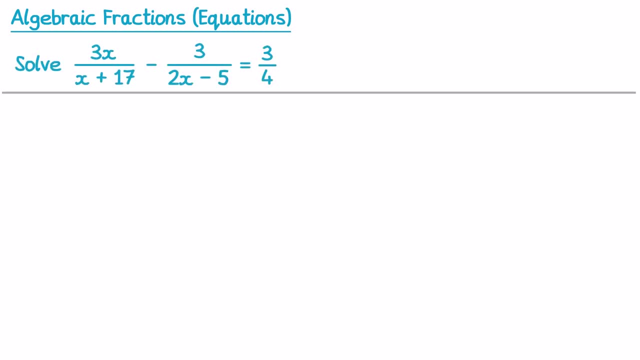 Now we're going to look at one more final question, This one here. We're going to start this one how we started all of the previous questions: We're going to write the left hand side over a common denominator, So for this one it'll be the product of x plus 17 and 2x minus 5.. 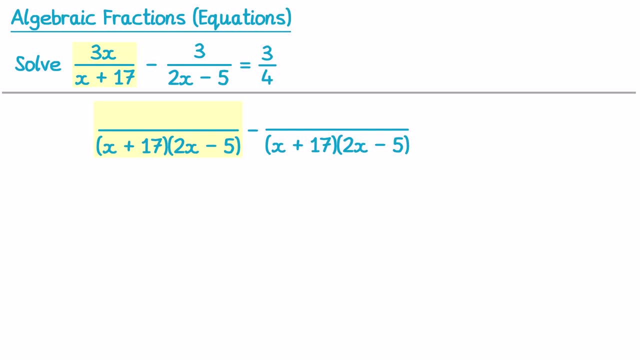 So if we compare these first two fractions, you can see we've multiplied by 2x minus 5.. So if we multiply by 2x minus 5 on the top we get 3x lots of 2x minus 5.. And for the right fractions, when we compare these, we've multiplied by x plus 17, so we need 3 lots. 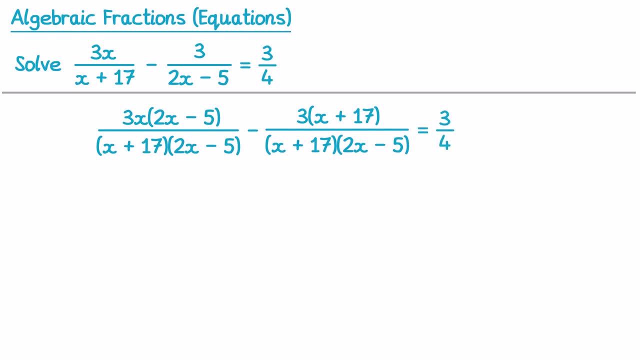 of x plus 17, and the right hand side is equal to 3 over 4.. Now we have that common denominator, we have 3x, and then brackets 2x minus 5. Then we have a subtraction in between them and 3x plus 17.. 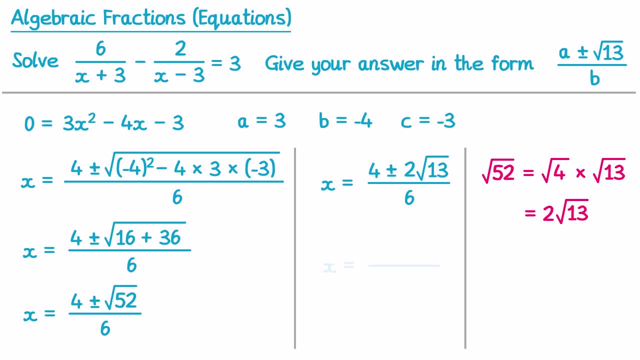 that is, we have a common factor of 2 here. If we divide all the terms by 2, we get x equals. If we divide the 4 by 2, we get 2.. Divide 2 root 13 by 2, you get 1 root 13.. Divide 6 by 2, you get 3.. This answer now matches the form we 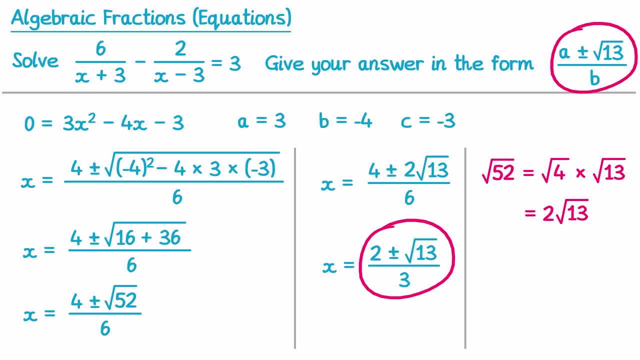 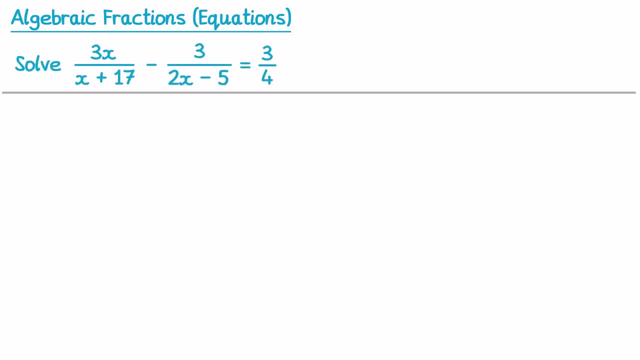 were asked in the question. You can see the value of a is 2 and the value of B is 3.. Now we're going to look at one more final question, This one here. We're going to start this one how we started all of the previous questions: We're 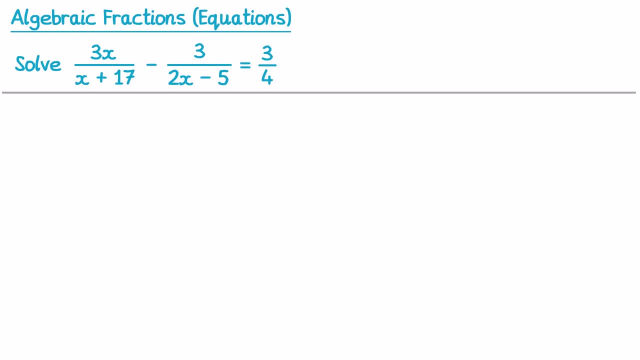 going to write the left-hand side over a common denominator. So for this one it will be the product of x plus 17 and 2x minus 5.. So if we compare these first two fractions, you can see we've multiplied by 2x minus 5.. 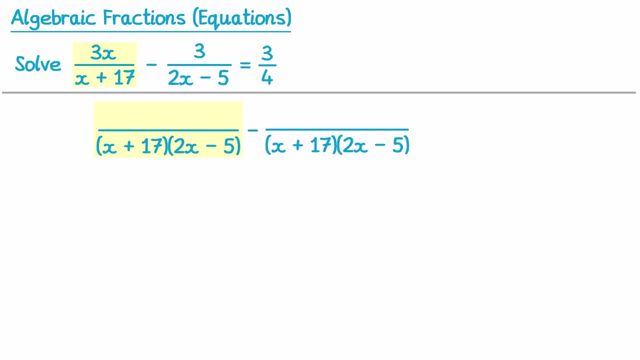 So if we multiply by 2x minus 5 on the top, we get 3x lots of 2x minus 5.. And for the right fractions, when we compare these, we've multiplied by x plus 17. so we need 3 lots of x plus 17.. And the right-hand side is equal to 3 over 4.. Now 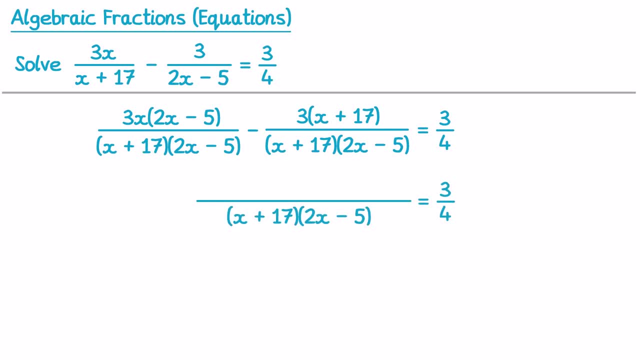 we have that common denominator. we can write them as one big fraction. So we've got 3x, and then brackets, 2x minus 5.. Then we have a subtraction in between them and 3x plus 17.. Next we're going to expand out that numerator, so we'll write: 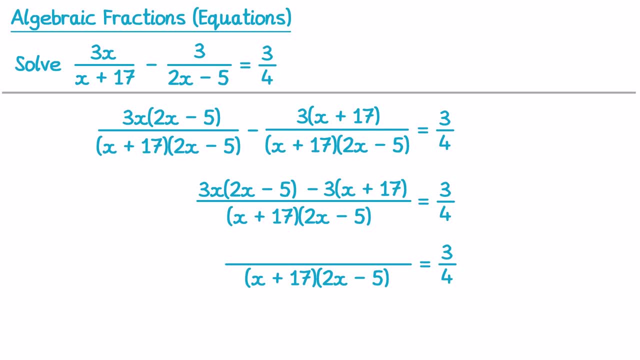 everything else the same. We have 3x multiplied by 2x, that's 6x squared 3x times negative 5, that's negative, 15x. Negative 3 times x. negative 3x and negative 3 multiplied by positive 17 is negative 51.. 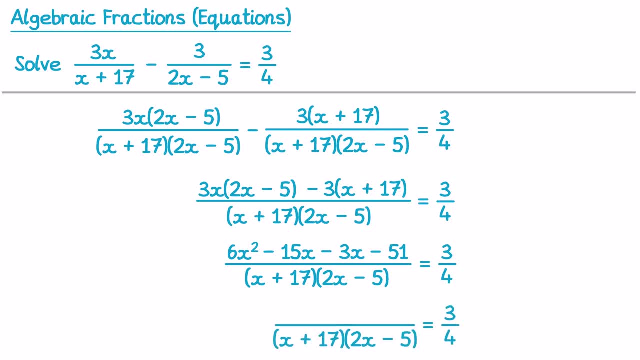 Now there's a little bit of simplifying we can do on the numerator. So we can't simplify the 6x squared- that's the only term with x squared. but we can simplify negative 15x subtract 3x, which is negative 18x, and then subtract 51. So 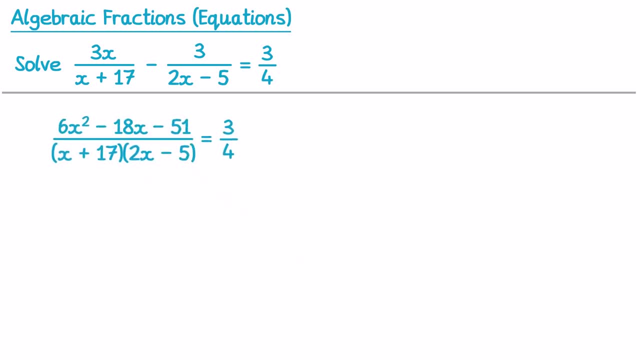 now we've written the left-hand side as a single fraction. What we're going to do next is multiply both sides by both of those brackets on that denominator. So if we multiply the left-hand side by x plus 17 and 2x minus 5, that will clear the 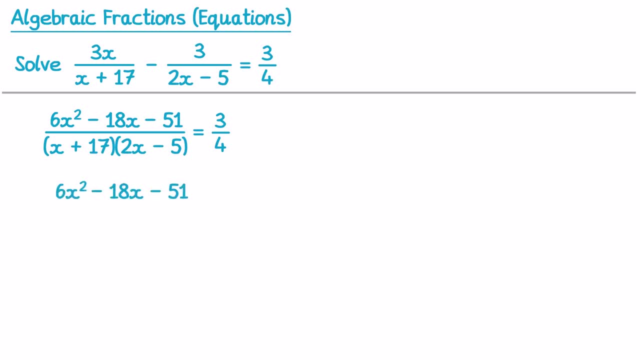 fraction. So we've got 6x squared minus 18x minus 51, and on the right-hand side we've got 6x squared minus 18x, minus 16x, minus 18x, minus 17x, minus 17 by 2x squared. 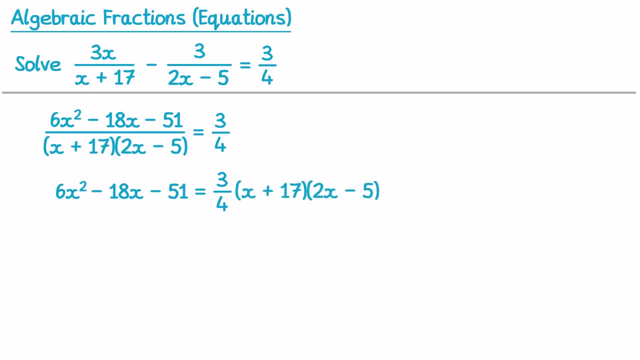 Now, in the previous couple of questions we haven't had to deal with a fraction like this on the right hand side. it was just an integer before those 2 brackets. To deal with this fraction, you can just multiply both sides by 4.. If we multiply the left-hand, 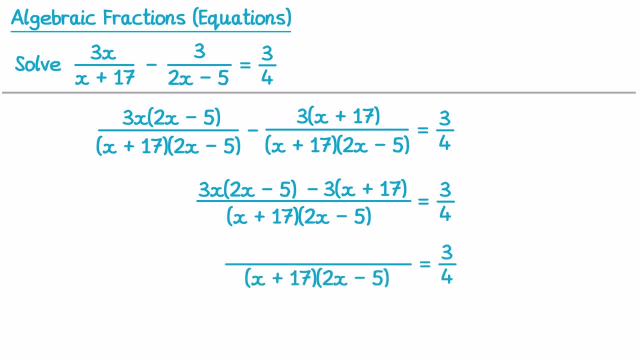 Next we're going to expand out that numerator, so we'll write everything else the same. We have 3x multiplied by 2x, that's 6x squared 3x times negative 5, that's negative 15x. Negative 3 times x, negative 3x and negative 3 multiplied by positive 17 is negative 51.. 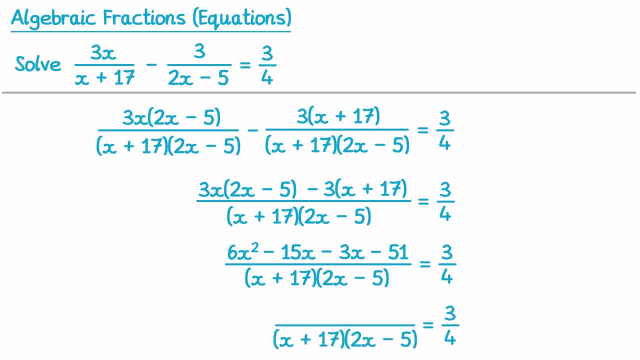 Now there's a little bit of simplifying we can do on the numerator. So we can't simplify the 6x squared- that's the only term with x squared- but we can simplify negative 15x, subtract 3x, which is negative 18x, and then subtract 51.. 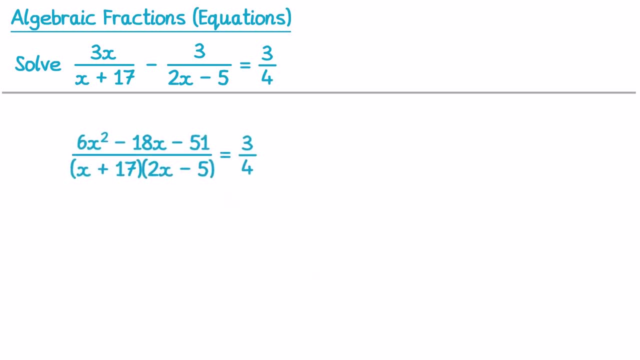 So now we've written the left hand side as a single fraction. What we're going to do next is multiply both sides by both of those brackets on that denominator. So if we multiply the left hand side by x plus 17 and 2x minus 5, that will clear the fraction. so we've got 6x squared minus 18x. 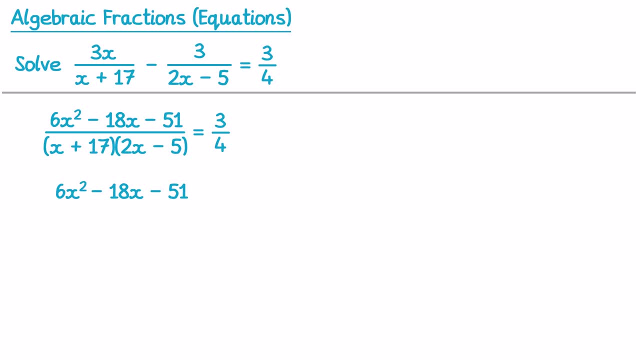 minus 51, and on the left hand side we've written 6x squared minus 18x minus 51.. On the right hand side we've just multiplied this 3 quarters by both of those brackets. Now, in the previous couple of questions we haven't had to deal with a fraction like this on the right. 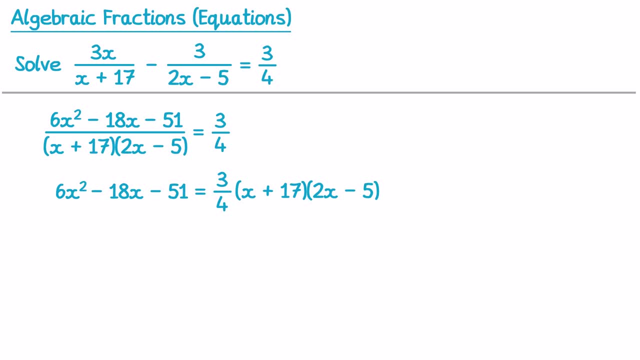 hand side. it was just an integer before those two brackets. To deal with this fraction, you can just multiply both sides by 4.. If we multiply the left hand side by 4, we get 4 lots of the left hand side, and if we multiply the right hand side by 4, that 4 will cancel. so we've just got 3 lots of those. 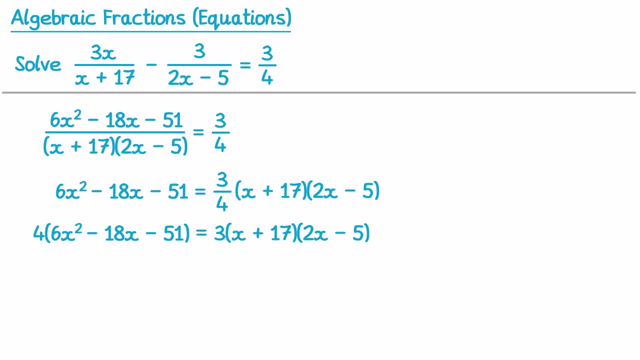 two brackets. Now we've got lots of expanding. to do so on the left hand side, we need to multiply by 4.. So we've got 4 lots of 6x squared- that's 24x squared. 4. lots of negative: 18x- that's negative. 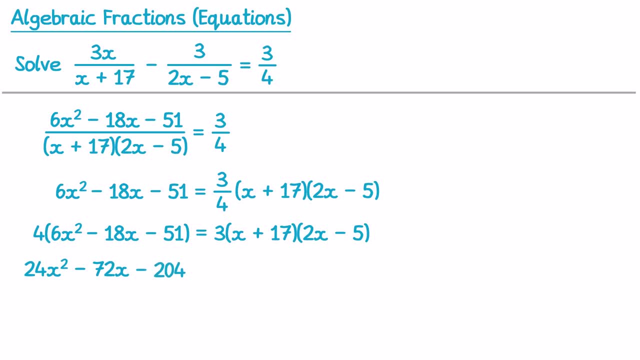 72x and 4, lots of negative. 51 is negative 204.. Then on the right hand side we're going to write a 3 and then a big bracket, then expand out the double bracket and write the terms inside this big bracket. So we've got x times 2x first, that's 2x squared. then we would do x times negative 5. 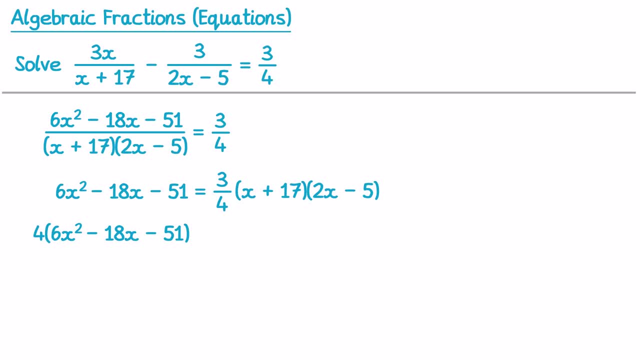 side by 4, we get 4 lots of the left-hand side, and if we multiply the right-hand side by 4, that 4 will cancel. so we've just got 3 lots of those 2 brackets. Now we've got lots of expanding to do So on the left-hand side we need to multiply. 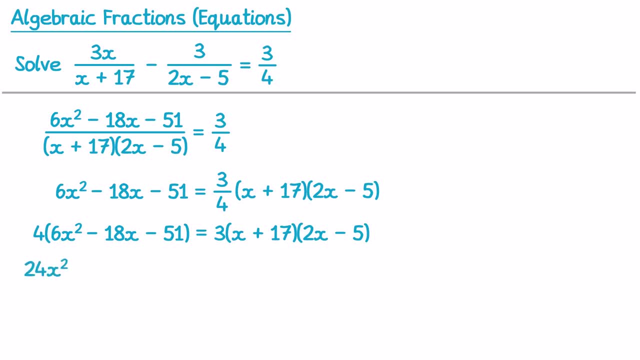 by 4.. So we've got four lots of 6x squared, that's 24x squared, four lots of negative 18x, that's negative 72x, and four lots of negative- 51 is negative 204.. Then on the right-hand side, 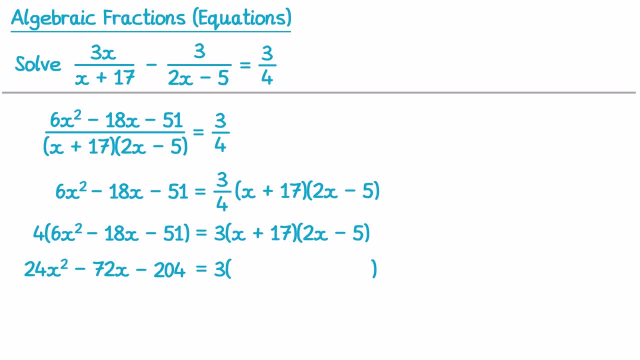 we're going to write a three and then a big bracket, then expand out the double bracket and write the terms inside this big bracket. So we've got x times 2x. first, that's 2x squared. Then we would do x times negative five, so negative 5x. 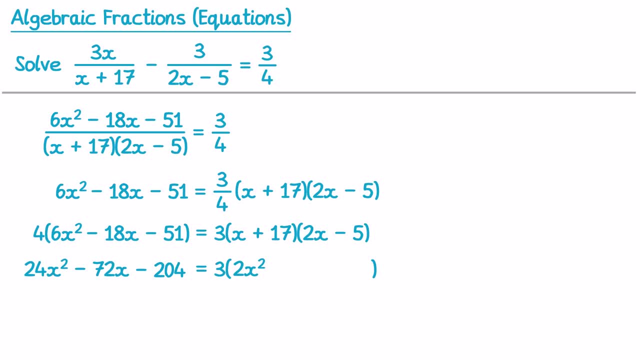 but we would also do 17 times 2x, which is a positive 34x. So we've got negative 5x plus 34x, that's positive 29x, And finally, 17 multiplied by negative five is negative 85.. 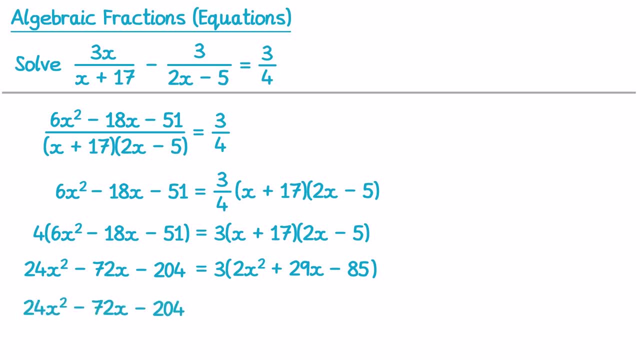 We can leave that left-hand side alone and expand this bracket on the right-hand side. We need to multiply by three, this time. Three lots of 2x squared is 6x. squared three lots of 29x is 87x. 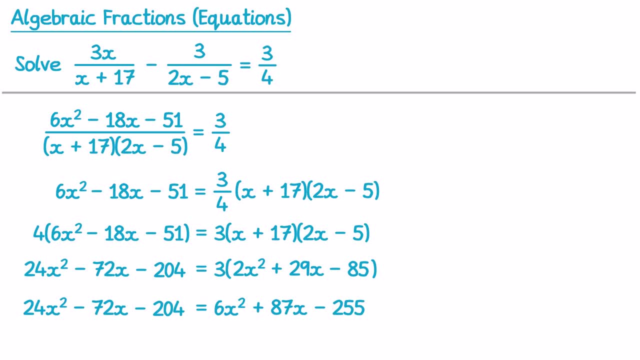 and three lots of negative. 85 is negative 255.. So we do end up with a quadratic equation to solve. Since we have more x squared on the left-hand side, I'm going to make the right-hand side equal to zero on this one. 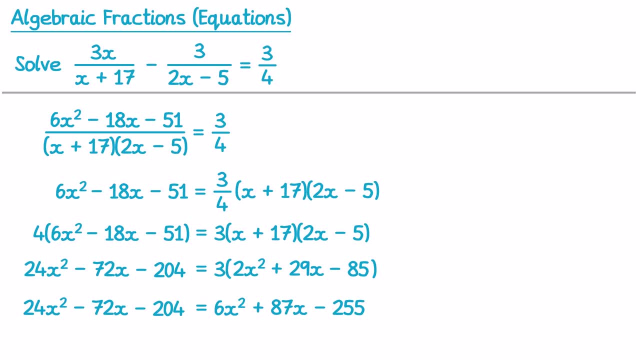 So I'd need to subtract 6x squared, subtract 87x and add 255 to both sides. So on the left-hand side, if I subtract 6x squared from 24x squared, I get 18x squared. And then if I subtract 87x from the 72x, 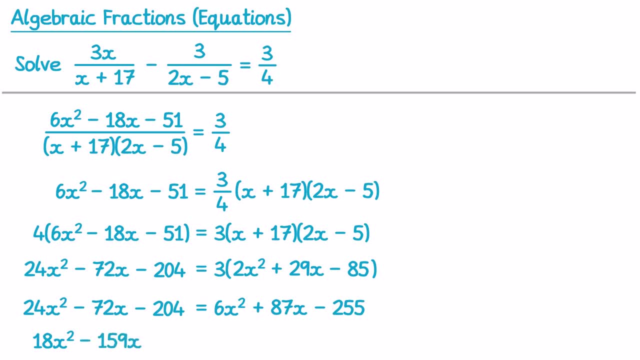 we get negative 159x, And then if we add 255 to negative 204, we end up with a positive 51. And the right-hand side, we know, will equal zero. Now let's take that quadratic equation and we're going to solve it. 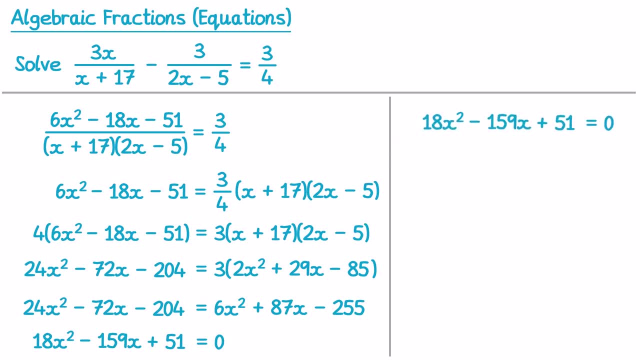 This one does look really nasty because of the size of the numbers, but there is actually a common factor of three here. If you divide 18x squared by three, you get 6x squared. Divide negative 159x by three, that's negative 53x. 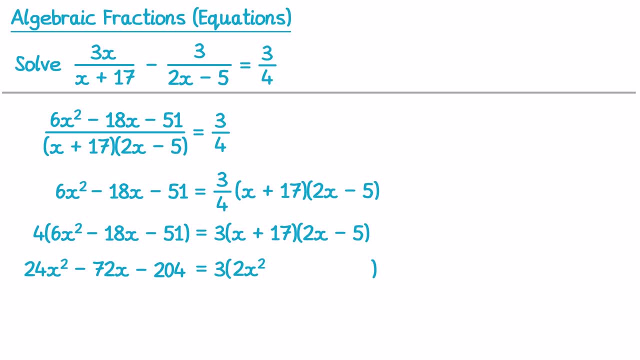 so negative 5x. but we would also do 17 times 2x, which is a positive 34x. So we've got negative 5x plus 34x, that's positive 29x and finally 17 multiplied by negative 5. 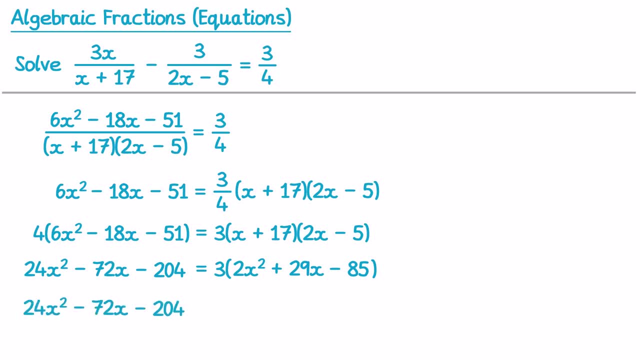 is negative 85.. We can leave that left hand side alone and expand this bracket on the right hand side. we need to multiply by 3. this time: 3 lots of 2x squared is 6x. squared 3 lots of 29x is 87x. 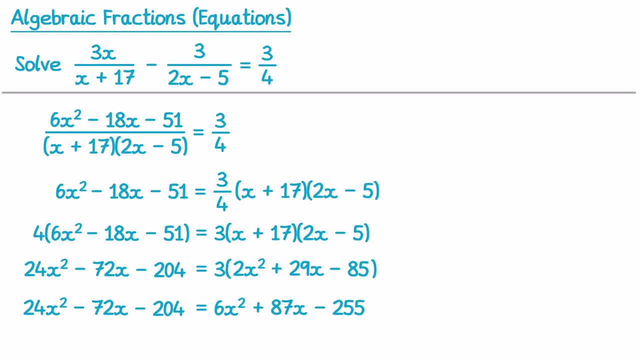 and 3, lots of negative. 85 is negative 255.. So we do end up with a quadratic equation to solve, Since we have more x squared, we can solve this by multiplying the two brackets by 3x squared On the left hand side. I'm going to make the right hand side equal to 0 on this one. 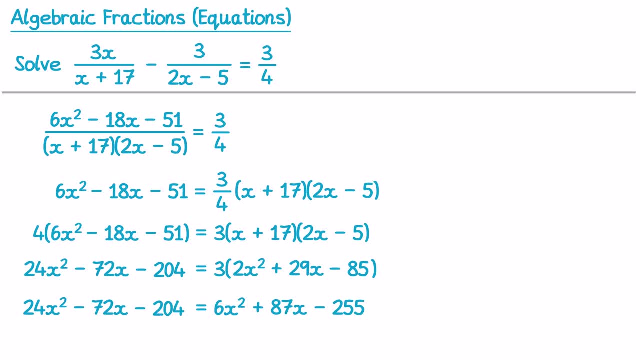 So I'd need to subtract 6x squared, subtract 87x and add 255 to both sides. So on the left hand side, if I subtract 6x squared from 24x squared, I get 18x squared, and then if I subtract 87x from the 72x, we get negative 159x. 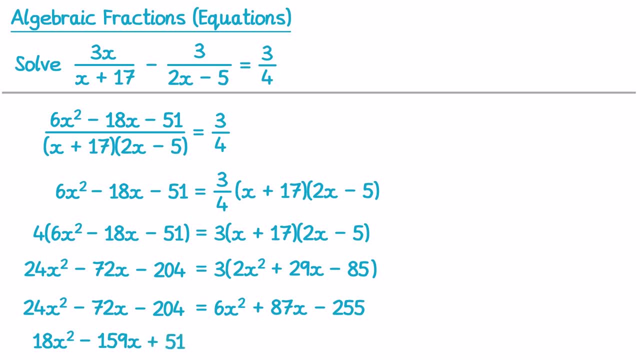 and then if we add 255 to negative 204, we end up with a positive 51 and the right hand side. we know we're going to have a 17 at the end. Now let's take that quadratic equation and we're going to solve it. This one does look really nasty because of the size of the numbers, but there is actually. 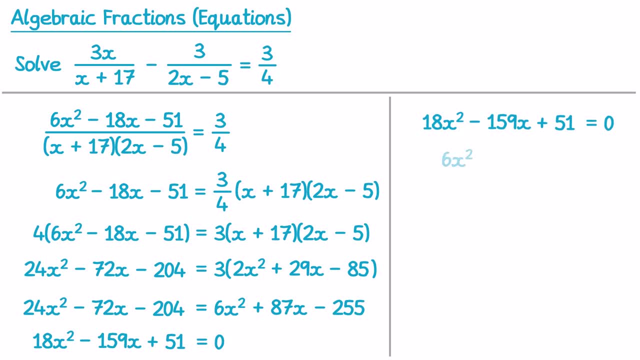 a common factor of 3 here. If you divide 18x squared by 3, you get 6x squared. divide negative 159x by 3, that's negative 53x, and divide the 51 by 3, that's 17.. And of course, if you divide 0 by 3, 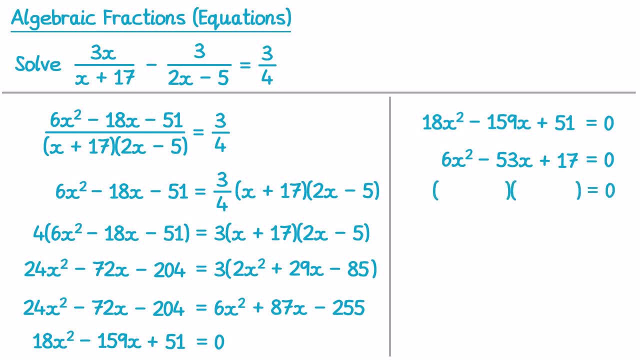 that's still 0. So we're going to factorise this one. actually, it will factorise into two brackets. Now it's actually quite fortunate we have a 17 at the end, Since we have a 17,. that's a prime number. we know its factors are only 1 and 17.. 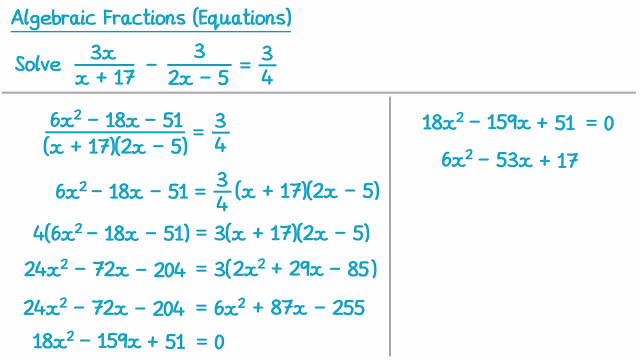 And divide the 51 by three, that's 17.. And of course, if you divide zero by three, that's still zero. So we're going to factorize this one. actually It will factorize into two brackets. Now, it's actually quite fortunate. 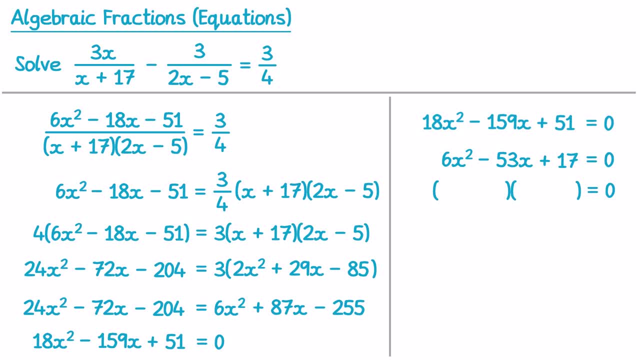 we have a 17 at the end. Since we have a 17, that's a prime number. we know its factors are only one in 17.. So if it did factorize, the only possible numbers we could put at the end of these brackets would be one in 17.. 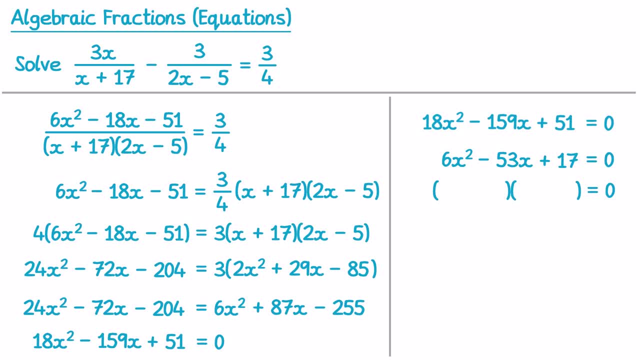 And they would actually both be negative as well, Since a negative times. a negative gives you a positive, so we still get a positive 17,. but the only way we'd end up with a negative 53x is if we had negative terms here. 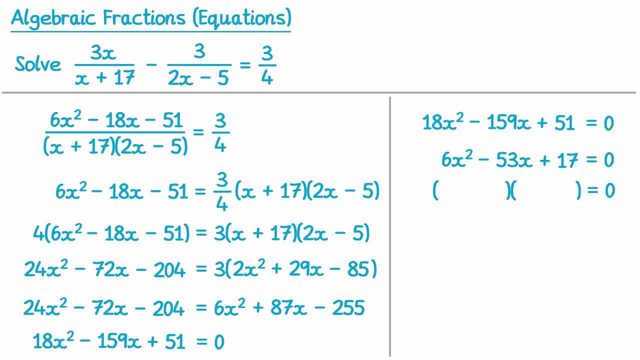 So if it did factorise, the only possible numbers we could put at the end of these brackets would be 1 and 17, and they would actually both be negative as well, Since a negative times a negative gives you a positive, so we still get a positive 17. 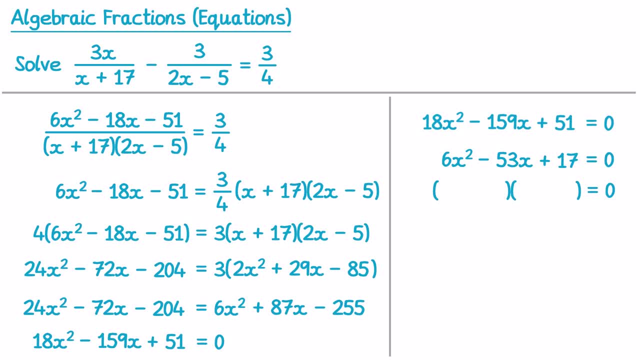 but the only way we'd end up with a negative 53x is if we had negative terms here. If they were both positive, that 53x wouldn't be attainable. So we can put negative 17 and negative 1 in these brackets, and then we just need to think about a few of the different. 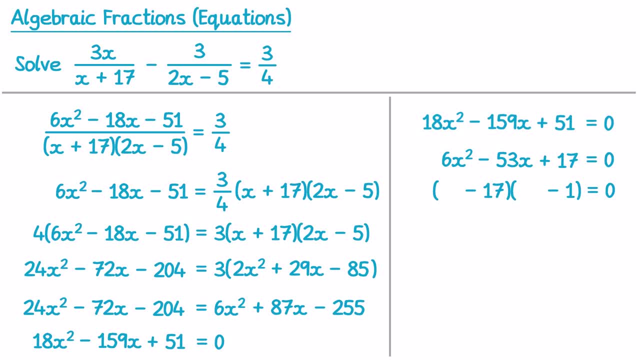 combinations here, So we can put negative 17 and negative 1 in these brackets, and then we just need to think about a few of the different combinations here to try and get that 6x squared. So we're either going to use a 6x and a 1x. 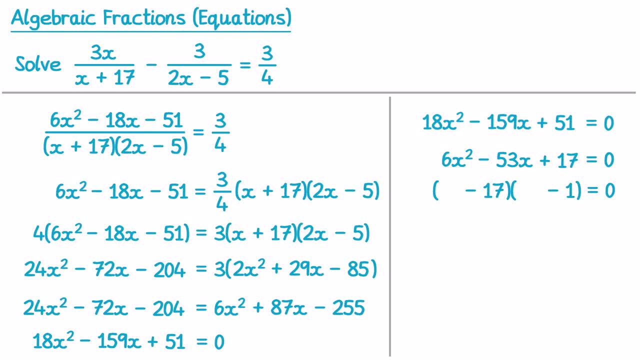 or a 3x and a 2x. Now, if you try a few different combinations out, it shouldn't take you too long to realise we need 2x minus 17 and 3x minus 1.. If you want, give this a go and expand it out.